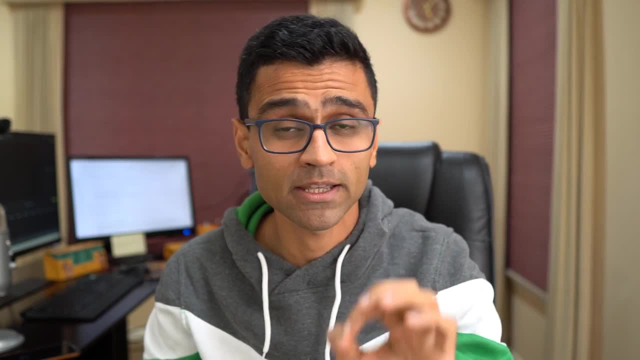 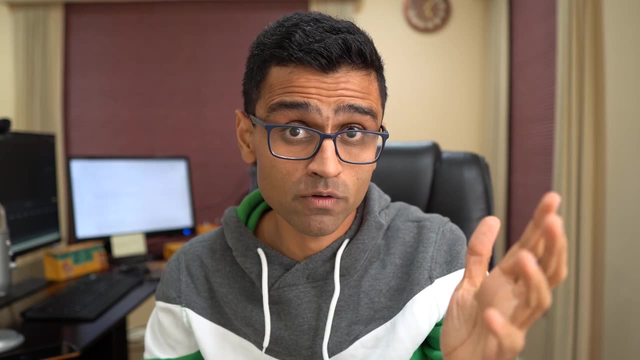 Overfitting is a very common issue in the field of machine learning, and L1 and L2 regularizations are some of the techniques that can be used to address the overfitting issue. In this video we'll go over some theory on what exactly L1 and L2 regularization is. 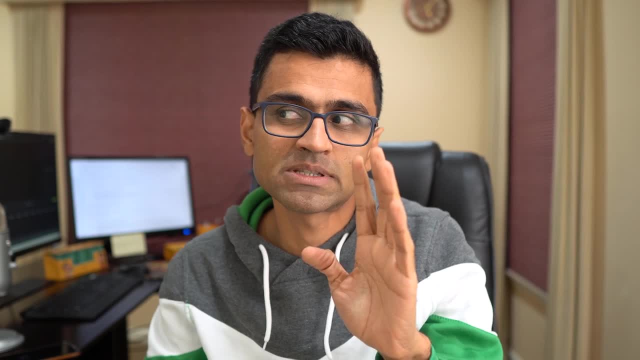 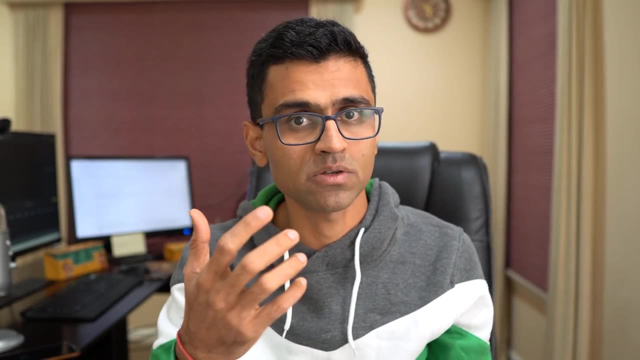 and then we'll write a python code and we'll see how a model which is an overfit can be addressed and the accuracy can be improved when you use L1 and L2 regularization. We will be using a housing price data set from the city of Melbourne. 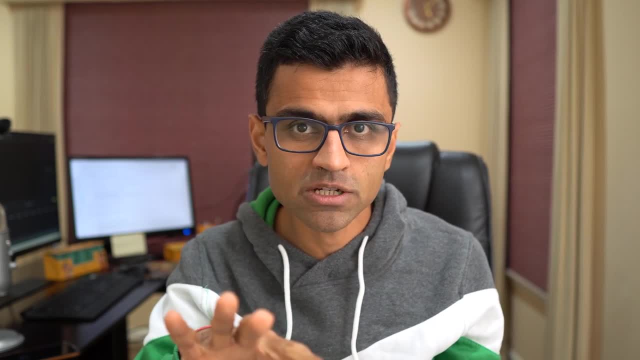 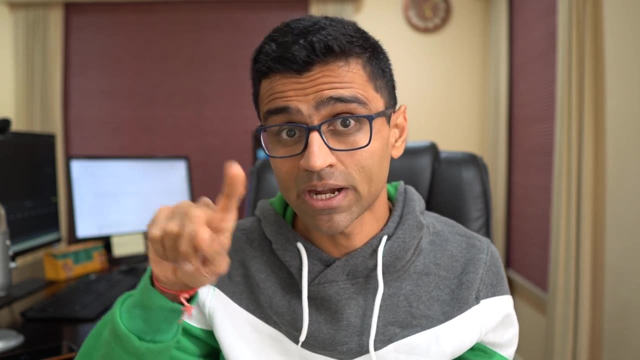 and we'll first build a model using a simple linear regression and we'll see it is overfitting the model, and then we'll use L1 and L2 regularization and we'll see how we address that overfitting issue and how it improves the score on our test set. So let's get started. 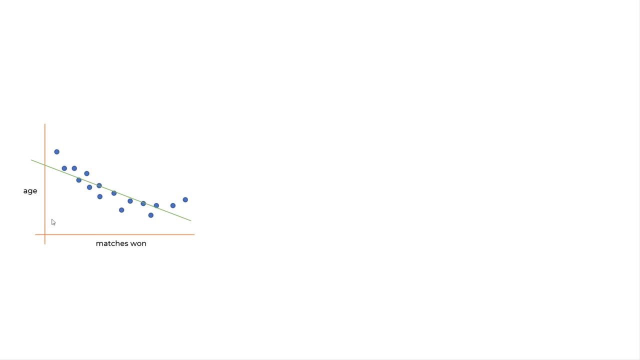 Let's say you're trying to predict number of matches won based on the age. Now, usually when the player gets aged- any sports person or athlete gets aged- the matches won kind of reduces. So you can have this kind of distribution where to build a model? you can create a simple. 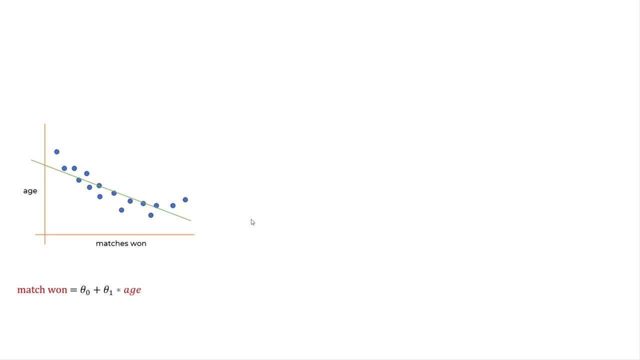 linear regression model and the equation might look like this: So matches won will be theta zero plus theta one and into age. So theta zero and theta one are just a constant. This is a regular linear, like simple linear equation. But you see that this line is not really accurately describing all the data points. 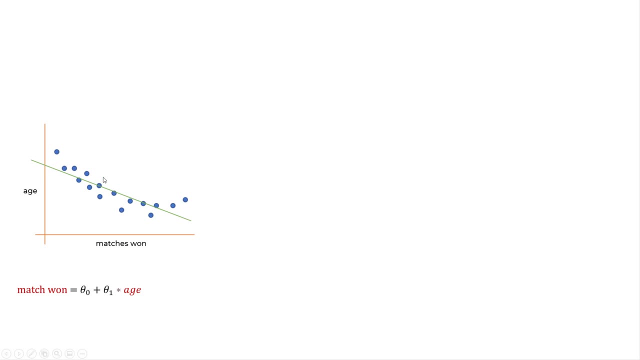 It is trying to find a best fit in terms of a straight line, but you see, all these data points are kind of going away, and then if you have test data points which are lying somewhere here, then this is not a very, very accurate representation of our data distribution. 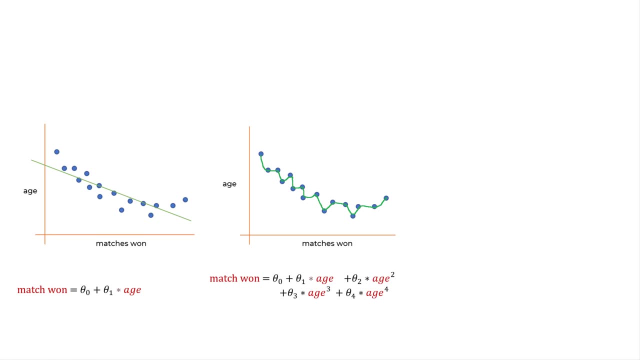 Then you can build a distribution which might look like this. So here we are trying to draw a line which kind of exactly passes through all our data points, and in that case your equation might look like this. So it's a higher order, higher order polynomial equation. 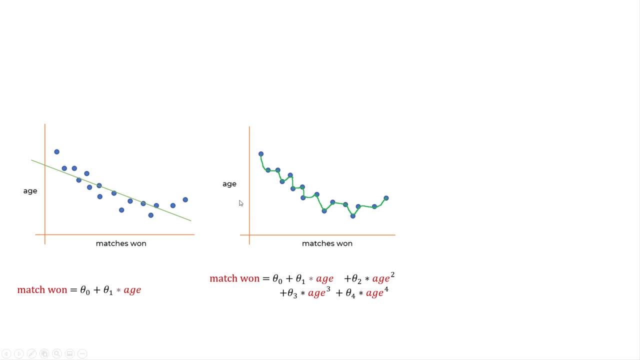 where you are trying to find out the matches won based on the age of a of a person. But here the issue is. this equation is really complicated. The line is a zigzag type of line which is just passing through all the data points. And now, if you have some general data points at the top, here again. 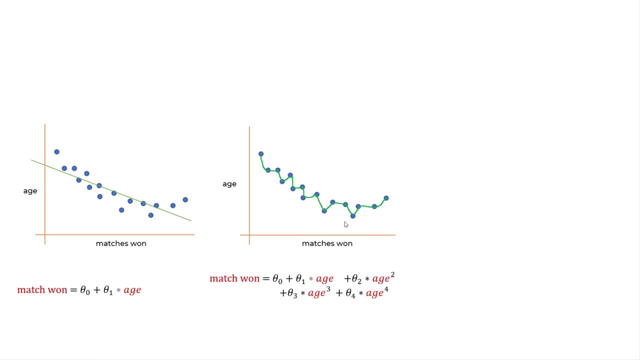 this is not generalizing the distribution really well. What might be better is if you have a line like this- So this is a balance between these two cases that we saw previously- So you can have, you know, only theta two into a square. The line will look like a curve and it can generalize your. 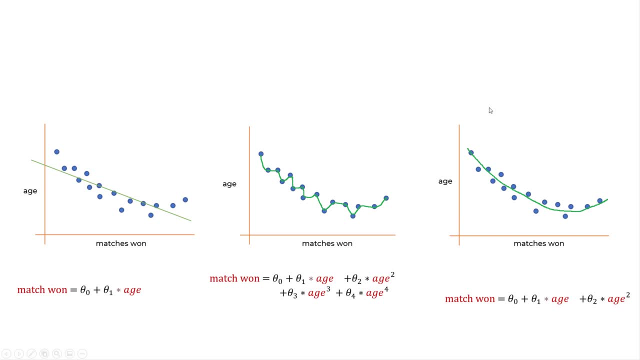 data point really well So that tomorrow, if new data point comes in this equation will be able to make a better prediction for you. So the first case is called underfitting, The second case is called overfitting and the third case is balance fit. So you kind of get an idea on overfitting here. 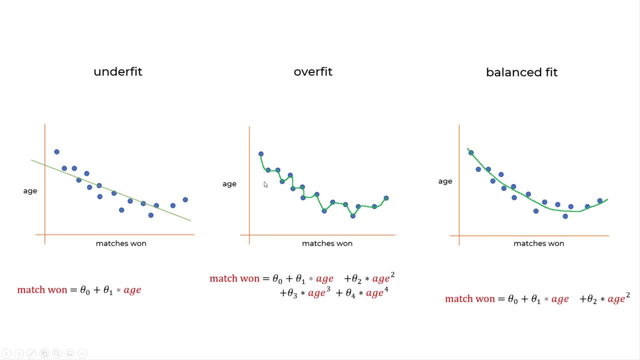 where if you try to run a training too much and try to fit too much to your training data set, then you will have issues with testing data set. When you try to predict your new data points, it might not do a better prediction, So you always have to keep a. 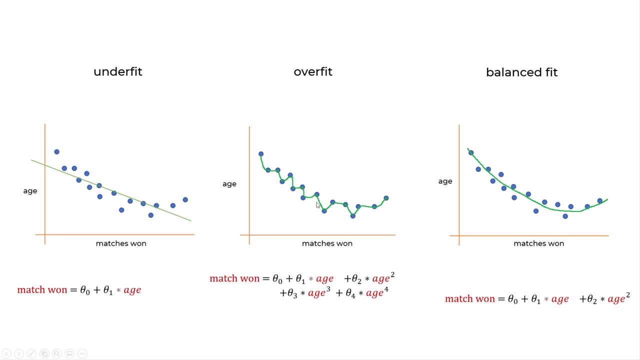 balance between these two extreme cases. Now, if you don't know about all these equations and everything, please refer to my linear regression tutorials I had in the same playlist. I had first few videos on linear regression, so you should watch that. That's kind of a prerequisite. 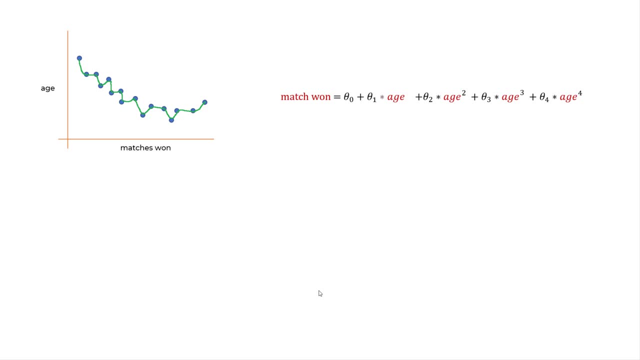 Now, how do you reduce overfitting? So here is my overfit line along with the equation. and if, in this equation, I somehow make sure that my theta zero and theta four is almost close to zero, then I will get an equation like this. So just think about: 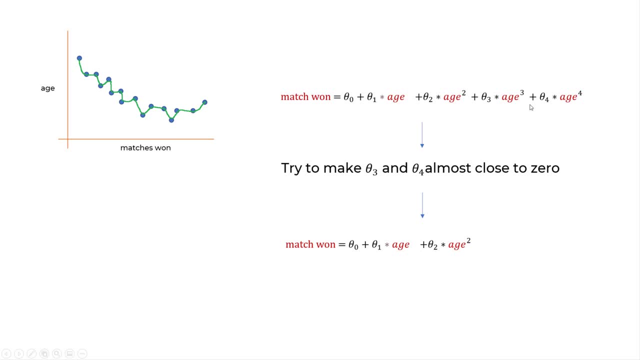 it. If theta three and theta four is almost close to zero, then you're kind of ruling out this whole factor and then you can create this type of equation. So the idea here is to shrink your parameters, Your parameters, which is theta zero, your overfitting line and then your overfitting. 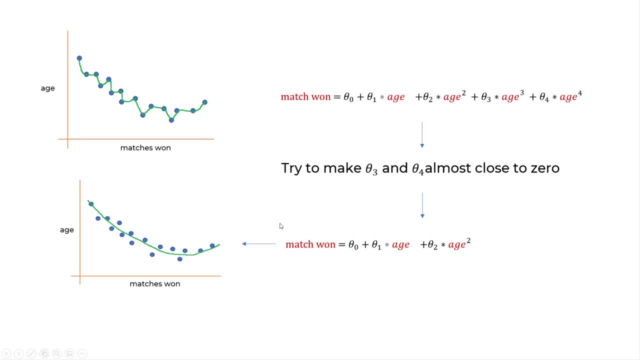 theta 3, theta 4, even theta 2, theta 1, if you can reduce this parameter, if you can keep these parameters smaller, then you can get a better equation for your prediction function. now, how do we do that? we earlier saw in our linear regression video that we calculate mean squared error. so when we run training we 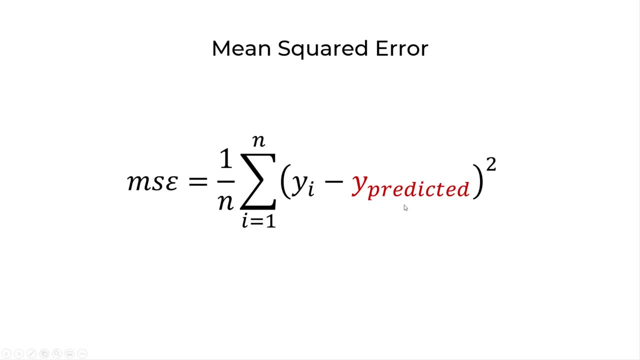 pass first sample and then we calculate Y predicted on some randomly initialized weights, then we compare it with the truth value and then this is how we call calculate mean squared error or MSE. here Y predicted is actually H theta XI, where H theta XI could be higher order. polynomial equation like this: okay, 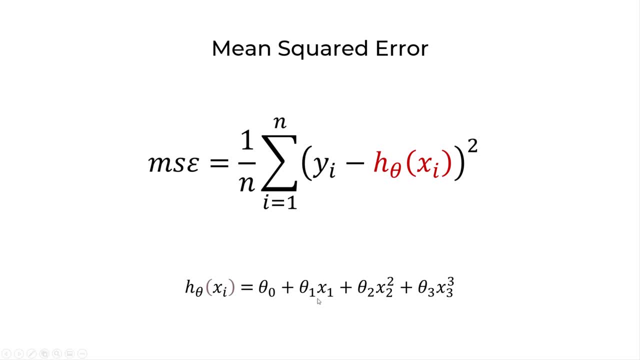 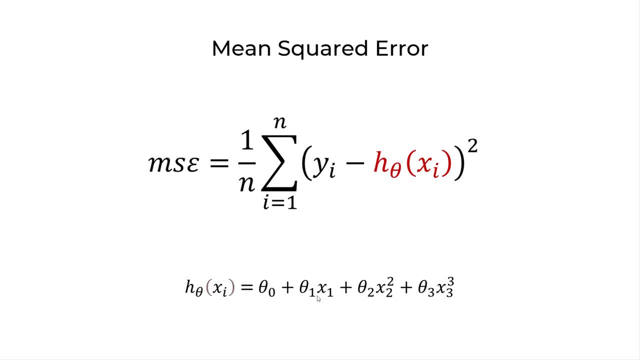 so in our case, it will be age of. so, in our case, it will be age of a person. if you have to talk thinking a person, if you have to talk thinking a person, if you have to talk thinking about housing price prediction, it will about housing price prediction, it will. 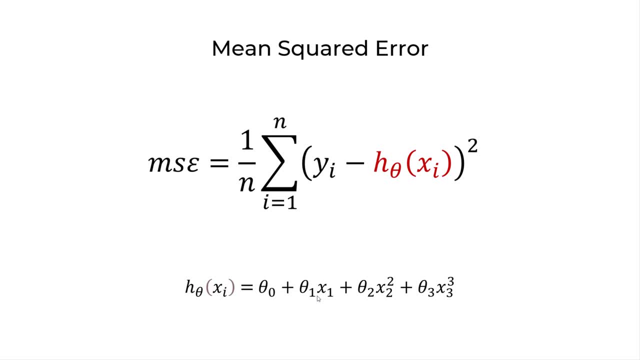 about housing price prediction. it will be the size of the house. now just think. be the size of the house now, just think. be the size of the house now. just think that in your mean square error function, that in your mean square error function, that in your mean square error function. so, by the way, this mean square error. 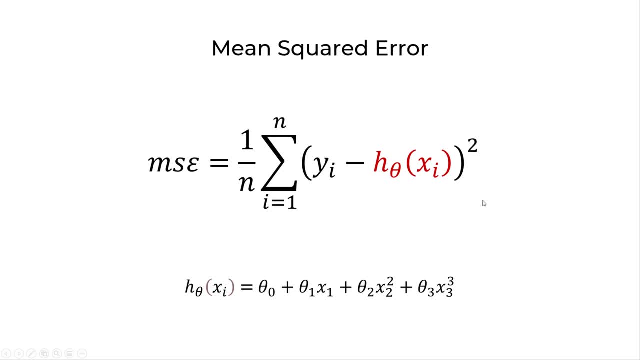 so, by the way, this mean square error. so, by the way, this mean square error. function we use during training and we function, we use during training and we function, we use during training and we want to minimize the value of this, this want to minimize the value of this, this. 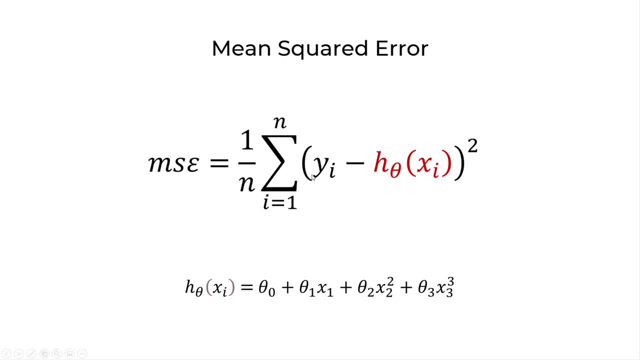 want to minimize the value of this. this error, you know on each iteration. so in error, you know on each iteration, so in error, you know on each iteration. so in this equation, what if I add this, this equation? what if I add this, this equation? what if I add this particular parameter? so what is this? so particular parameter. so what is this? so, particular parameter, so what is this? so there is this lambda which is a free. there is this lambda which is a free. there is this lambda which is a free parameter. you can control it. it's like a parameter, you can control it. it's like a. 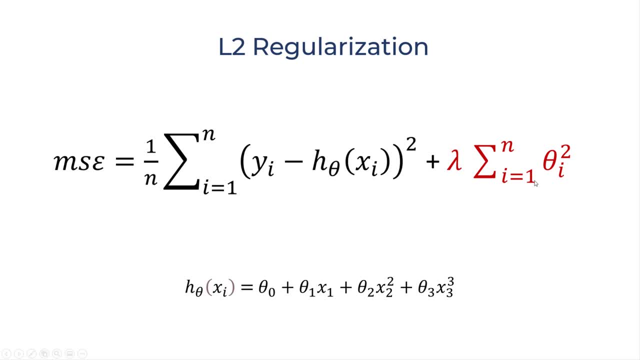 parameter. you can control it. it's like a tuning knob and you are making a square tuning knob and you are making a square tuning knob and you are making a square of each of these theta parameters. so now, of each of these theta parameters. so now of each of these theta parameters. so now, if your theta gets bigger, this value. 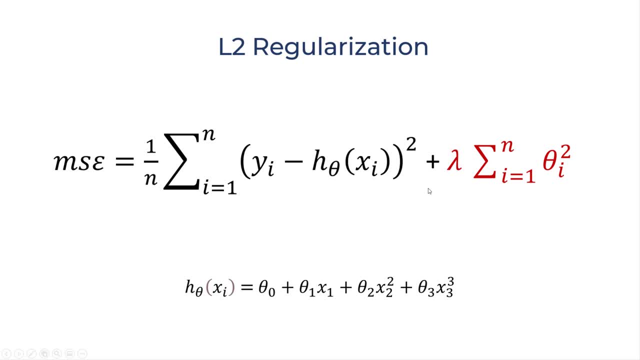 if your theta gets bigger, this value, if your theta gets bigger, this value will get bigger, the error will be big. will get bigger, the error will be big. will get bigger, the error will be big. you know and your model will not. you know and your model will not. 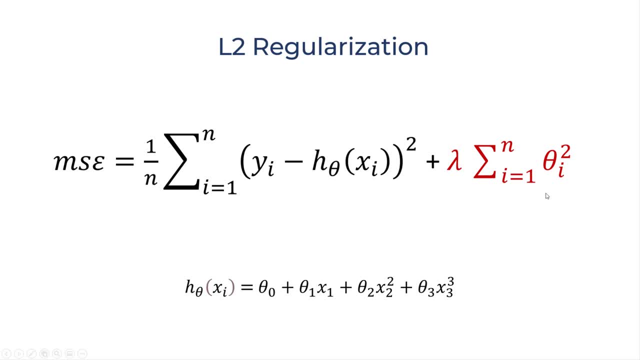 you know and your model will not convert. so essentially what you're doing, convert. so essentially what you're doing. convert so essentially what you're doing is you are penalizing higher values of is. you are penalizing higher values of is. you are penalizing higher values of theta here. so whenever model tries to 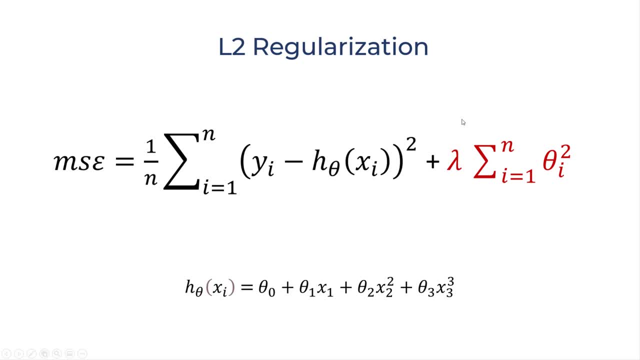 theta here. so whenever model tries to theta here, so whenever model tries to make the theta value higher, you are make the theta value higher. you are make the theta value higher. you are adding a penalty here. so by adding this, adding a penalty here, so by adding this. 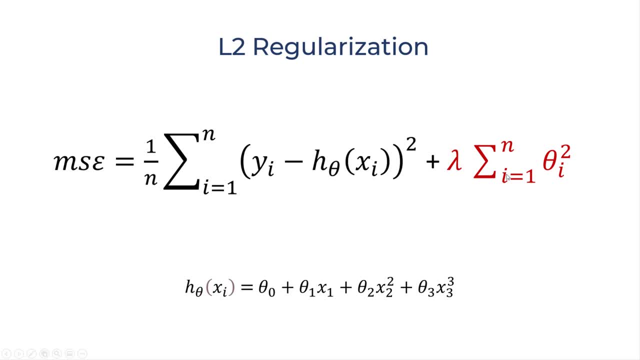 adding a penalty here. so by adding this penalty, you're making sure your theta penalty, you're making sure your theta penalty, you're making sure your theta value doesn't go too high. so they will value doesn't go too high. so they will value doesn't go too high. so they will remain very small. you can fine-tune this. 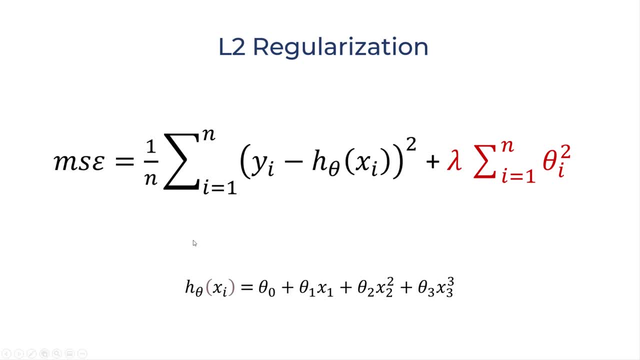 remain very small. you can fine-tune this, remain very small. you can fine-tune this thing using this, this parameter lambda thing. using this, this parameter lambda thing. using this, this parameter lambda here, and if you make this bigger the here, and if you make this bigger the. 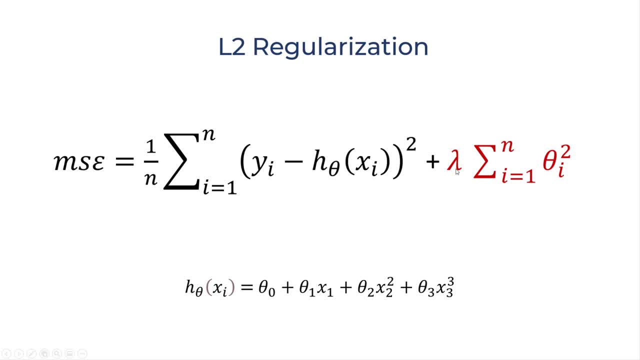 here, and if you make this bigger, the theta value will even get smaller and theta value will even get smaller, and theta value will even get smaller and smaller. you know, and if you get this smaller, you know, and if you get this smaller, you know, and if you get this smaller, than theta value can be bigger. so 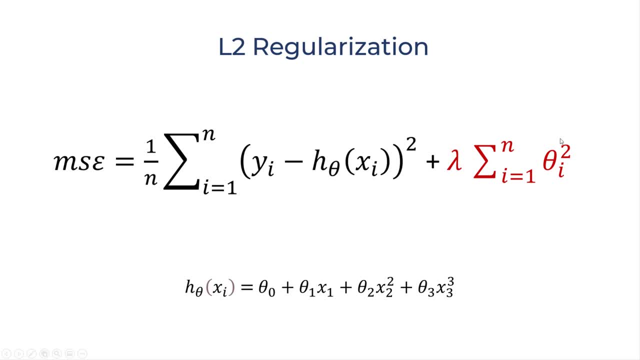 smaller than theta value can be bigger. so smaller than theta value can be bigger. so this is called l2 regularization. it is. this is called l2 regularization. it is. this is called l2 regularization. it is called l2 because we are using the called l2 because we are using the. 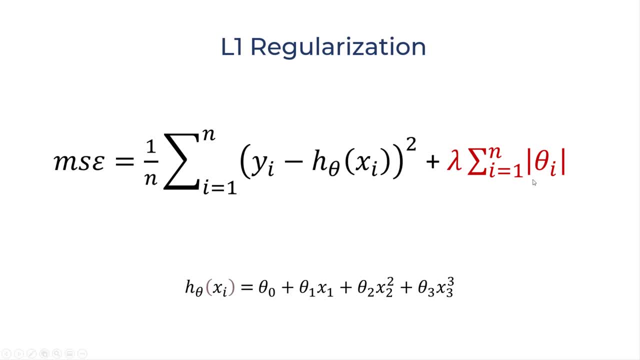 called l2 because we are using the square, and in l1 regularization you are square and in l1 regularization you are square and in l1 regularization you are using the absolute value. so that is the using the absolute value. so that is the using the absolute value. so that is the only difference between l1 and l2. that 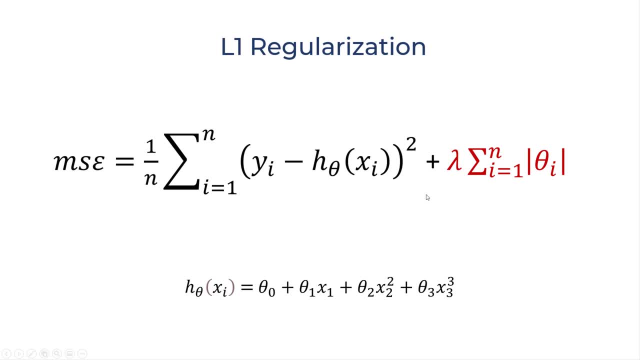 only difference between l1 and l2, that only difference between l1 and l2. that in l1 you are using absolute value of. in l1 you are using absolute value of. in l1 you are using absolute value of theta parameter. here again, if theta is. 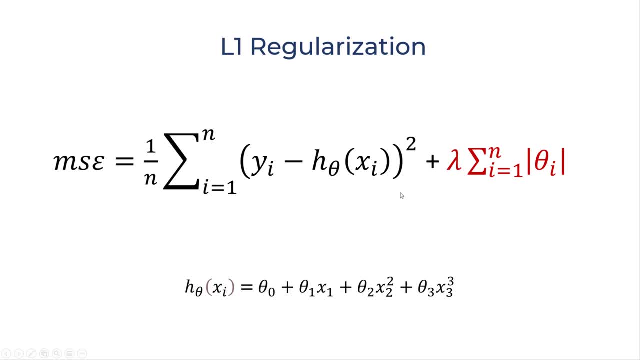 theta parameter here again. if theta is theta parameter here again, if theta is bigger, the error overall error is big, bigger the error overall error is big, bigger the error overall error is big and it kind of acts as a penalty so that and it kind of acts as a penalty so that 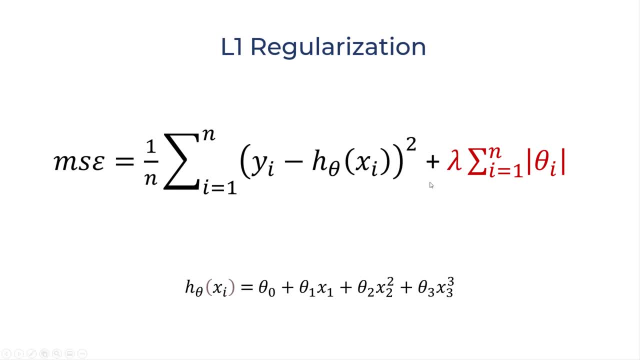 and it kind of acts as a penalty so that during your training overall, the value during your training overall, the value during your training overall, the value of theta will remain smaller and again of theta will remain smaller, and again of theta will remain smaller and again. going back to this equation here, when 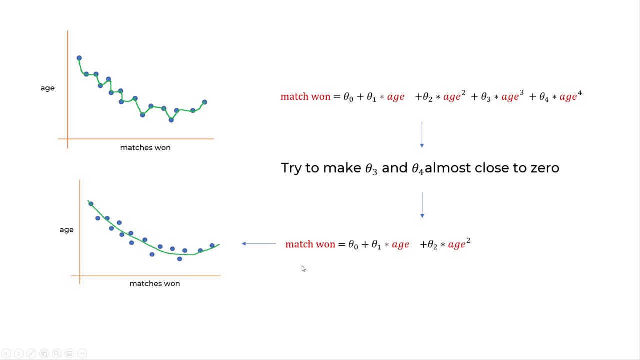 going back to this equation here, when going back to this equation here, when these values remain smaller, you come up. these values remain smaller. you come up, these values remain smaller. you come up with a simpler equation. you know you with a simpler equation. you know you with a simpler equation. you know you don't make it really complicated and 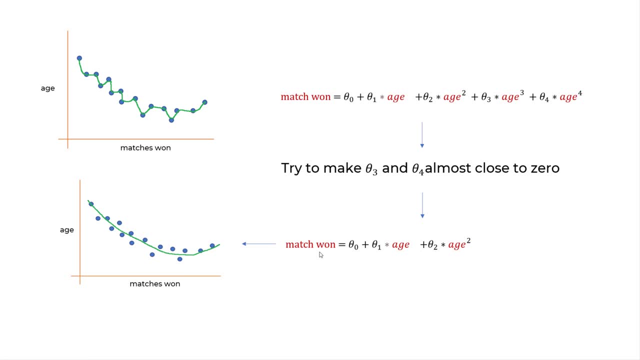 don't make it really complicated and don't make it really complicated and simpler equations are the best to simpler equations are the best to simpler equations are the best to represent the generic case of your represent, the generic case of your represent, the generic case of your prediction. alright, so let's get into. 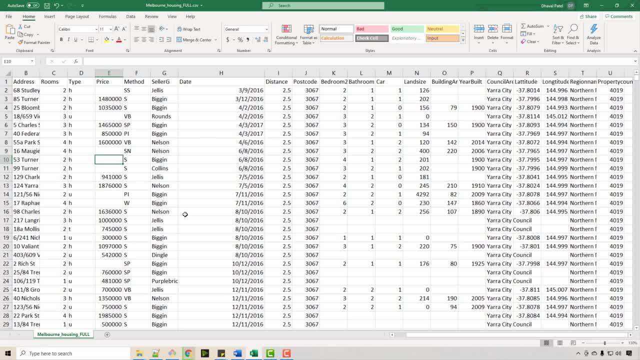 prediction. alright, so let's get into prediction. alright, so let's get into coding. now for the coding. I am using coding, now for the coding. I am using coding, now for the coding. I am using housing price data set for Melbourne City. housing price data set for Melbourne City. 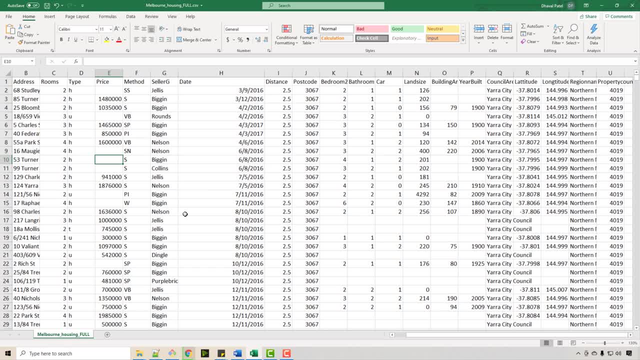 housing price data set for Melbourne City. I got this data set from Kegel and we. I got this data set from Kegel and we. I got this data set from Kegel and we are going to build a linear regression, are going to build a linear regression. 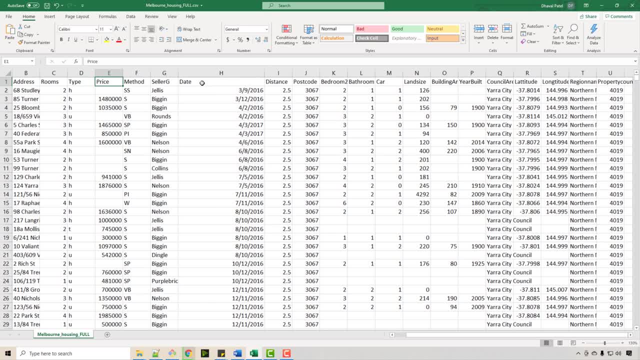 are going to build a linear regression model. so you can see that there are model. so you can see that there are model. so you can see that there are different features, such as room, the different features such as room, the different features such as room, the distance, postal code, bathroom, car and so. 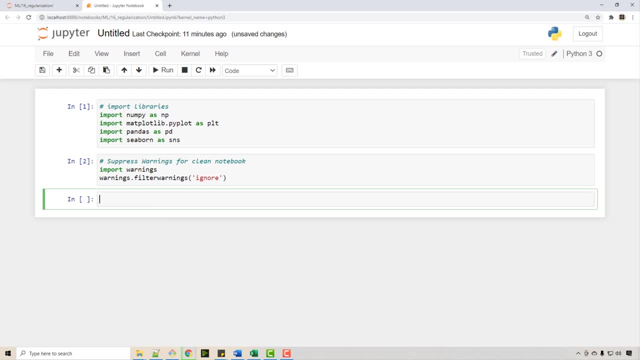 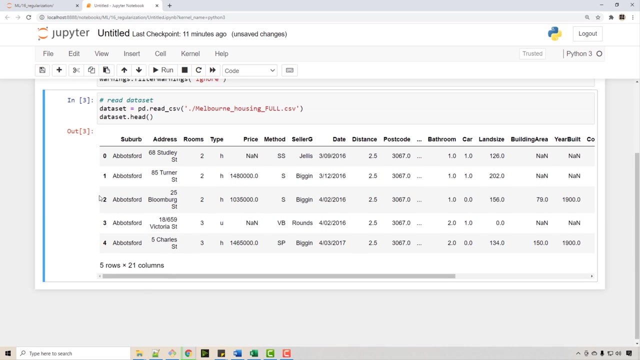 distance postal code- bathroom car, and so distance postal code, bathroom car, and so data set and just call it data set, data set, data set. you know, you know, you know. so I imported this into my data frame. so I imported this into my data frame. so I imported this into my data frame now and data frame is looking good. I'm. 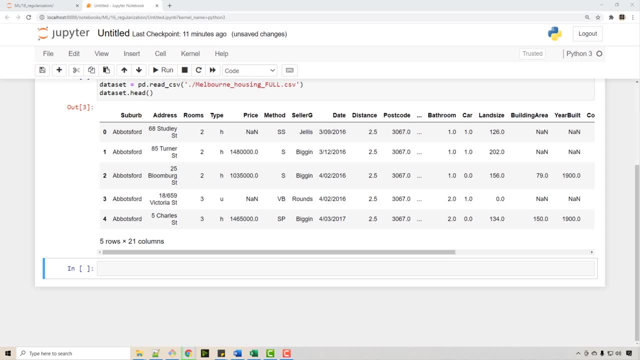 now and data frame is looking good. I'm now and data frame is looking good. I'm going to do some exploration of my data. going to do some exploration of my data. going to do some exploration of my data frame now and kind of print of value frame now and kind of print of value. 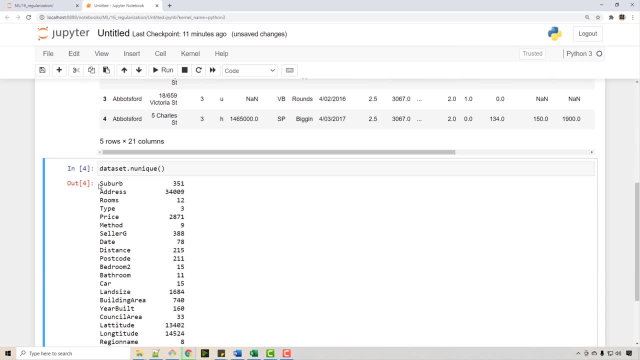 frame now and kind of print of value, unique values in data set. so you see unique values in data set. so you see unique values in data set. so you see like there are 351 suburbs, these many like there are 351 suburbs, these many like there are 351 suburbs, these many addresses, and so on. also, if you look at 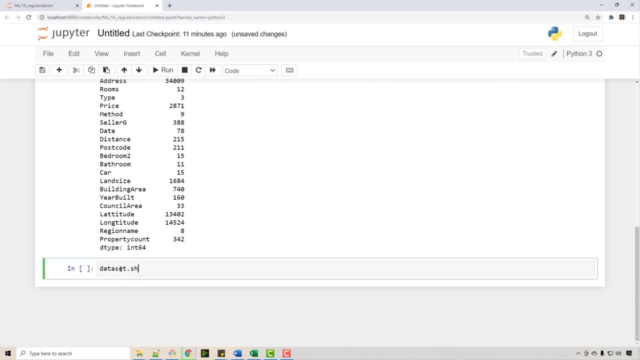 addresses and so on. also, if you look at addresses and so on, also if you look at the shape of the data set, there are three, four, eight, five is five. there are three, four, eight, five is five. there are three, four, eight, five is five. seven records and 21 columns in total. 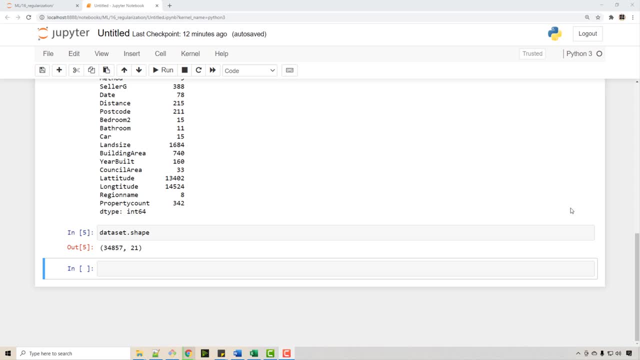 seven records and 21 columns in total: seven records and 21 columns in total. now I'm going to discard certain. now I'm going to discard certain. now I'm going to discard certain columns. I just did visual observation columns. I just did visual observation columns. I just did visual observation and discarded certain columns which I 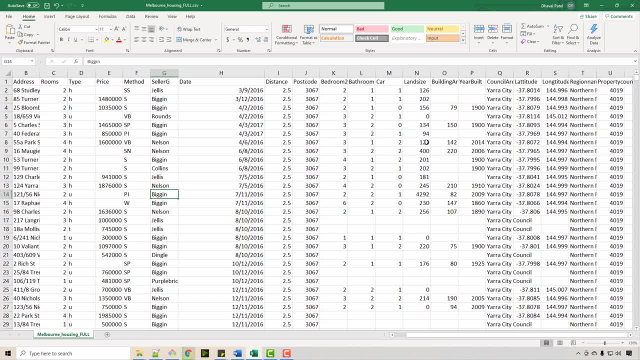 and discarded certain columns which I and discarded certain columns which I don't think are very useful, so for don't think are very useful, so for don't think are very useful. so, for example, date example, date example, date, right, so date is it's not useful, so I. 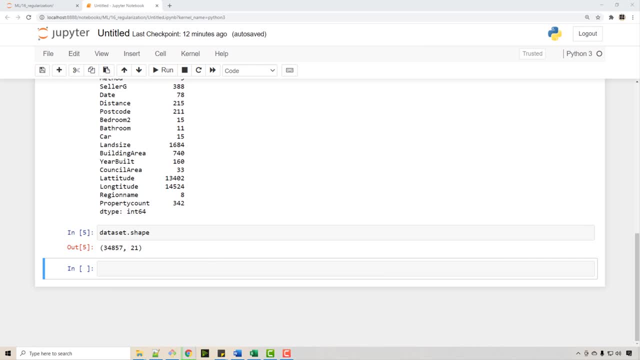 right, so date is it's not useful. so I right, so date is it's not useful. so I will just say, okay, here are the columns, will just say okay, here are the columns, will just say okay, here are the columns that are useful, that are useful, that are useful. and I'm just doing copy paste to save the. 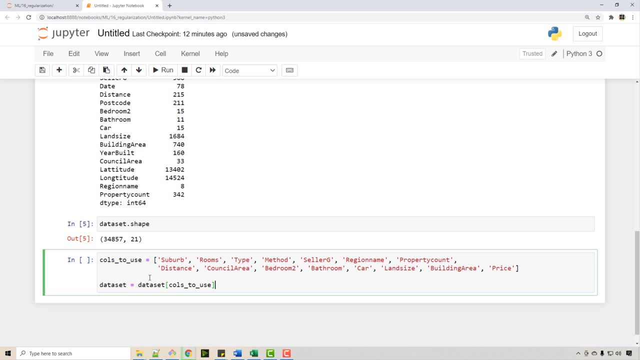 and I'm just doing copy paste to save the. and I'm just doing copy paste to save the time on recording. and when you pass time on recording, and when you pass time on recording and when you pass these columns to this data set, you get these columns to this data set, you get. 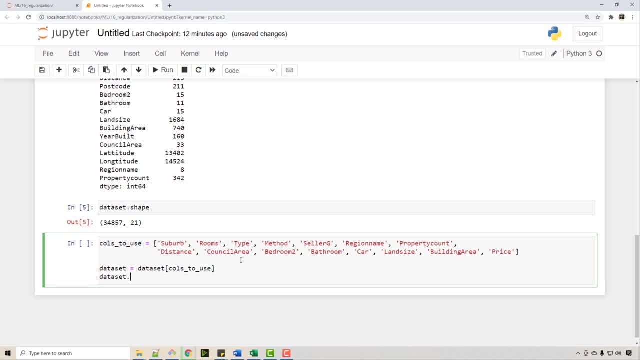 these columns to this data set. you get the filter data set okay, and then again the filter data set okay, and then again the filter data set okay, and then again you can run data set dot head. so now I. you can run data set dot head, so now I. 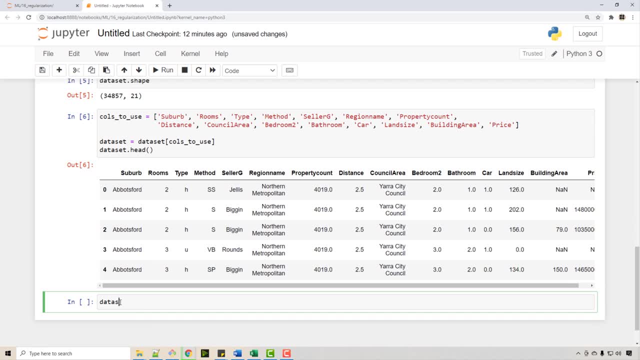 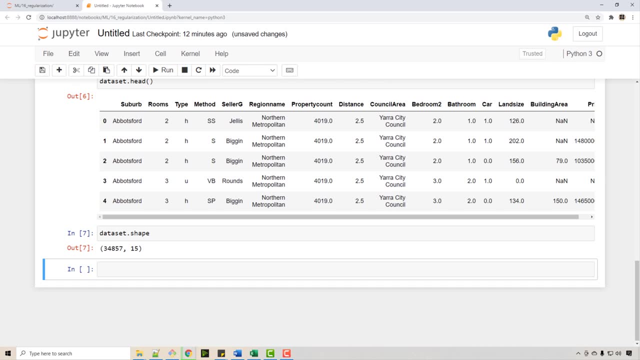 you can run data set dot head. so now I have less columns. okay. so if you do data, have less columns, okay. so if you do data, have less columns, okay. so if you do data, set dot shape, set dot shape, set dot shape, you know 15 columns instead of 21. 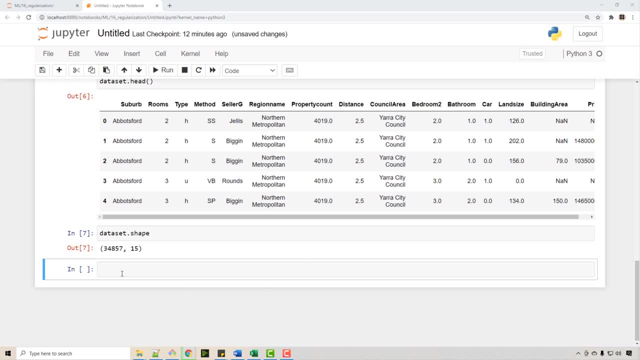 you know 15 columns instead of 21. you know 15 columns instead of 21. now I want to check for the any values. now. I want to check for the any values. now I want to check for the any values and you can do it by calling: is any? 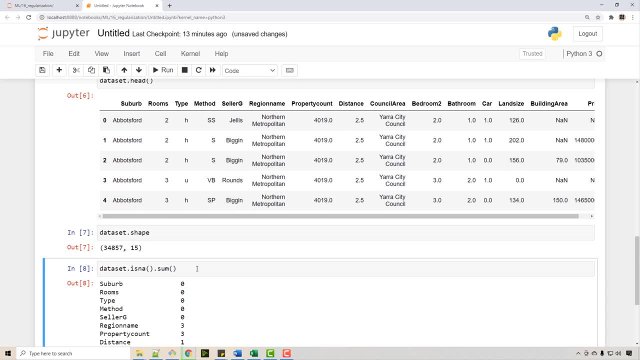 and you can do it by calling: is any? and you can do it by calling: is any function on your pandas data frame and function on your pandas data frame and function on your pandas data frame and you can do dot sum and it will tell you. you can do dot sum and it will tell you. 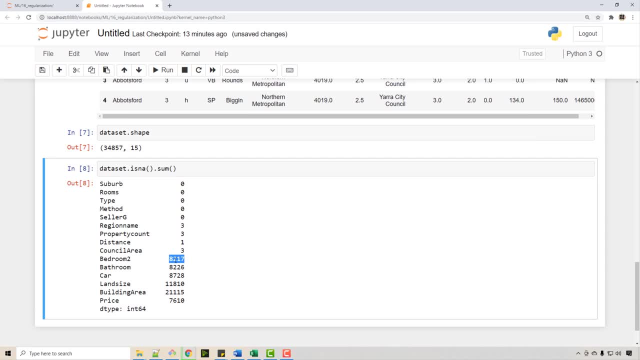 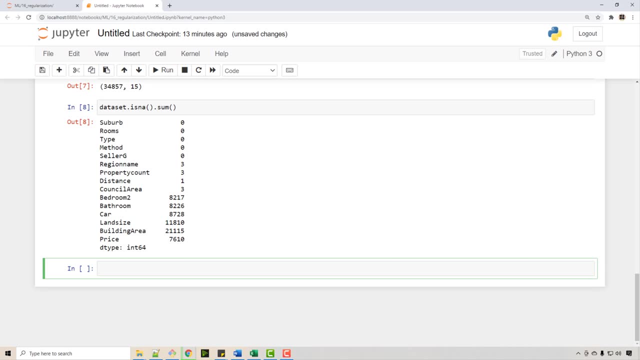 you can do dot sum and it will tell you so. bedroom 2 has total eight thousand. so bedroom 2 has total eight thousand. so bedroom 2 has total eight thousand two hundred and seventeen any values. you two hundred and seventeen, any values. you two hundred and seventeen, any values. you know any rows. so now we need to handle. 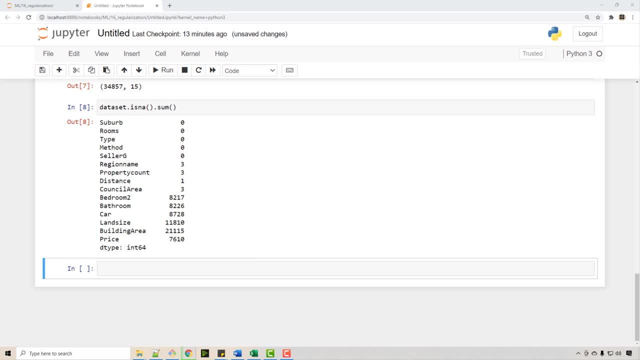 know any rows, so now we need to handle know any rows, so now we need to handle these rows. so I'm going to fill some of these rows. so I'm going to fill some of these rows, so I'm going to fill some of these columns with value 0, okay, and those. 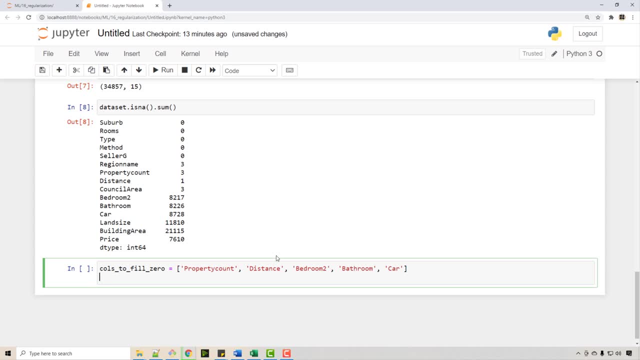 these columns with value 0, okay, and those, these columns with value 0? okay, and those columns, are these so columns to fill columns? are these so columns to fill columns? are these so columns to fill with 0? are this with 0? are this with 0? are this, for example, if car is any, which means 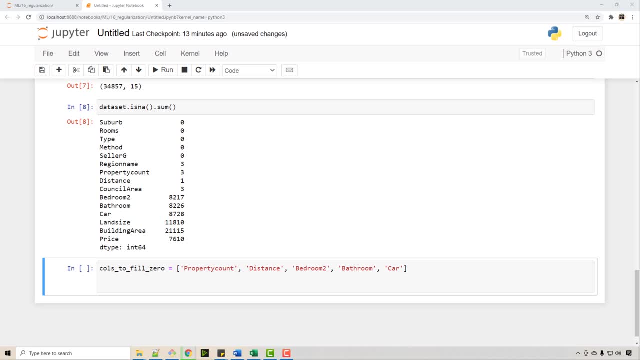 for example, if car is any which means, for example, if car is any which means you, you, you know there is no car parking available. know there is no car parking available. know there is no car parking available for that particular property and when for that particular property and when. 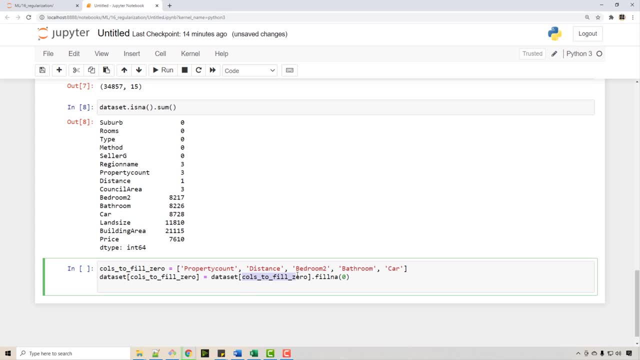 for that particular property. and when you run this function, so in your data you run this function, so in your data you run this function. so in your data set you're saying all these columns fill set, you're saying all these columns fill set. you're saying all these columns fill any with 0, it will take those any. 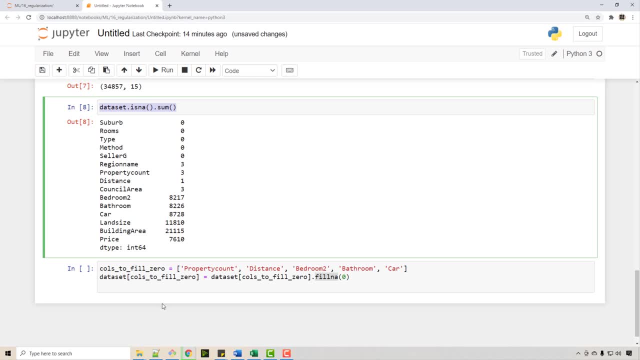 any with 0, it will take those. any. any with 0, it will take those any values and it will fill them with 0, so values and it will fill them with 0, so values and it will fill them with 0. so now, after doing this, I will do this. 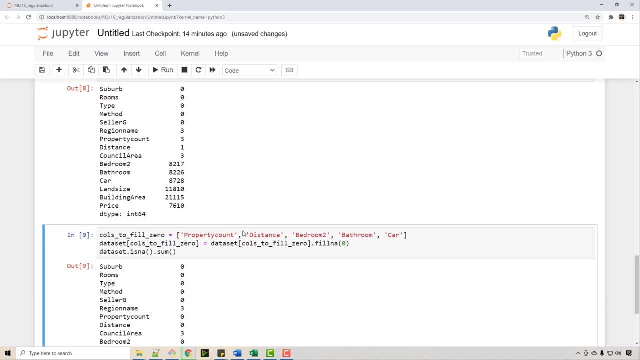 now, after doing this, I will do this, now, after doing this, I will do this again. and you can see that, for example, again. and you can see that, for example again. and you can see that, for example, property count: it was 3, so property. property count: it was 3, so property. 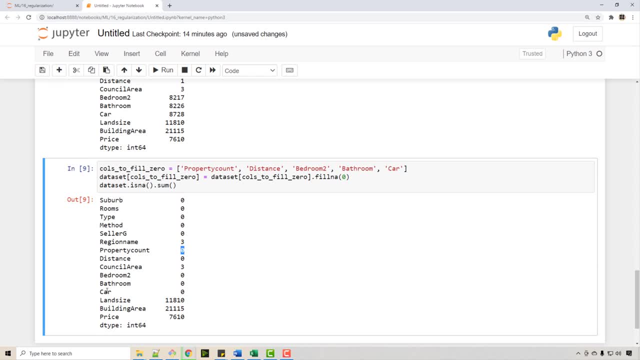 property count. it was 3, so property count now is 0. all the any values are count now is 0. all the any values are count now is 0. all the any values are filled similarly. car car parking there filled similarly car car parking. there filled similarly car car parking. there were 8,700 rows with any value. now I 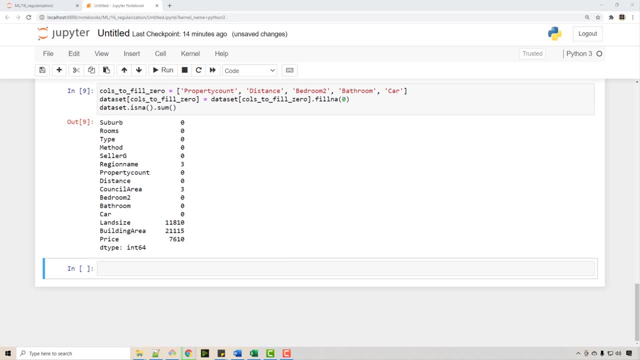 were 8,700 rows with any value. now I were 8,700 rows with any value. now I made it 0 now what we are going to do is: made it 0 now. what we are going to do is made it 0 now. what we are going to do is we'll look at certain other columns, such 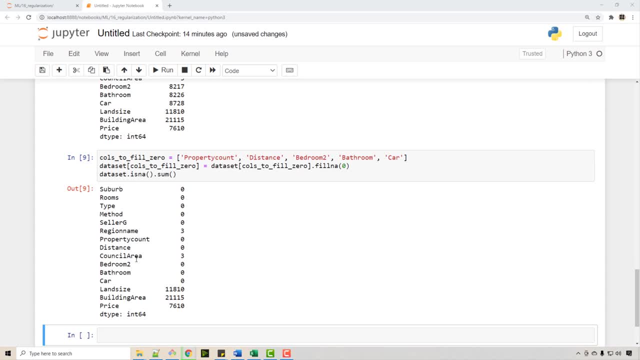 we'll look at certain other columns, such we'll look at certain other columns such as land size and building area, and we as land size and building area, and we as land size and building area, and we will like this true and we will will like this true and we will. 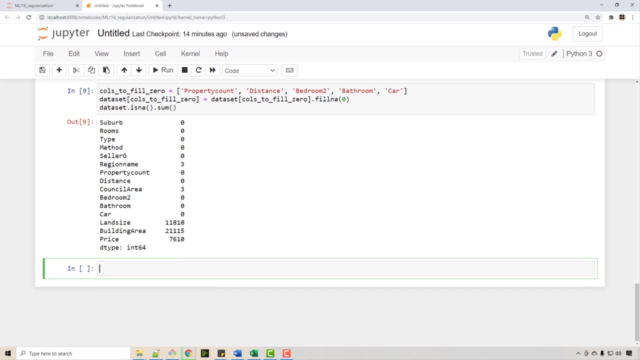 will like this. true, and we will calculate the mean and will fill those. calculate the mean and will fill those, calculate the mean and will fill those with the mean value. so the way you do with the mean value, so the way you do with the mean value, so the way you do that is using this function. so you are. 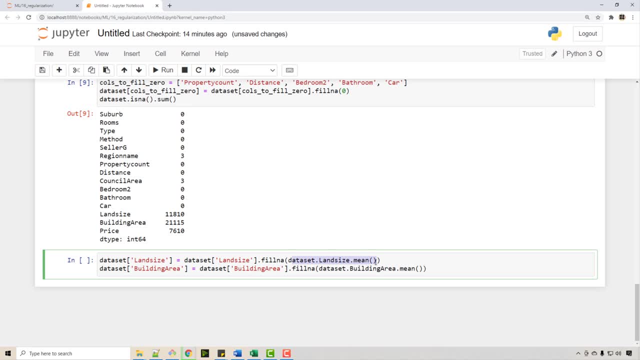 that is using this function. so you are. that is using this function. so you are doing: land size dot fill any with the doing land size dot fill any with the doing land size dot fill any with the mean of the same column. okay, so this is mean of the same column. okay, so this is. 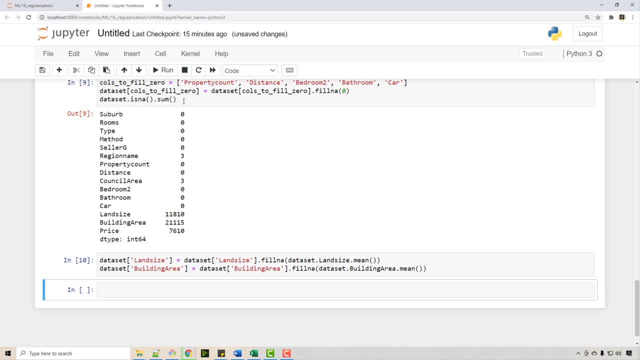 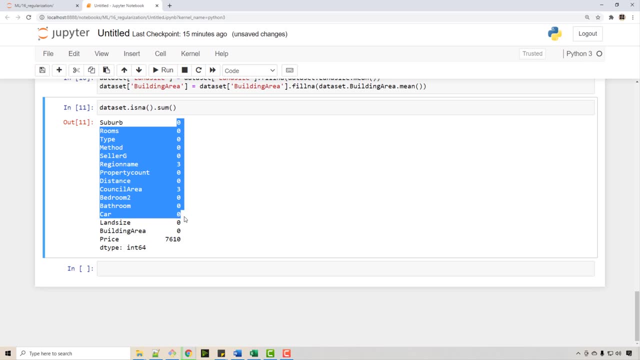 mean of the same column. okay, so this is a safe, safe assumption, and after that, a safe, safe assumption, and after that, a safe, safe assumption, and after that, when you do any, when you do any, when you do any, you find that you find that no values with zero, I mean there are. 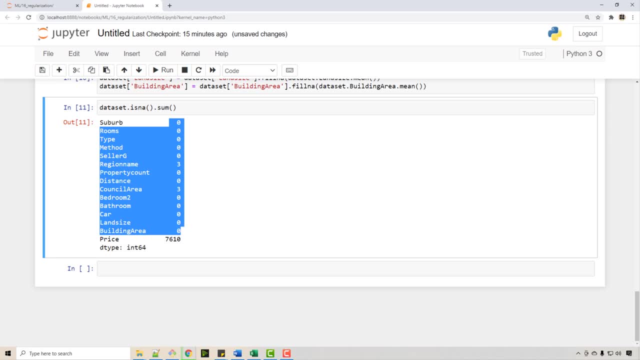 no values with zero. I mean there are no values with zero. I mean there are some prices, but if you look at your some prices, but if you look at your some prices, but if you look at your independent features there, that's that's. independent features there, that's that's. 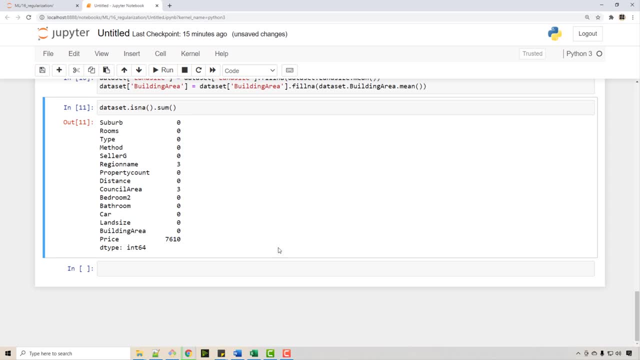 independent features there. that's that's basically now curated and there are basically now curated and there are basically now curated and there are. there are only two columns region name. there are only two columns region name. there are only two columns region name and this council leaders. I'm not going. 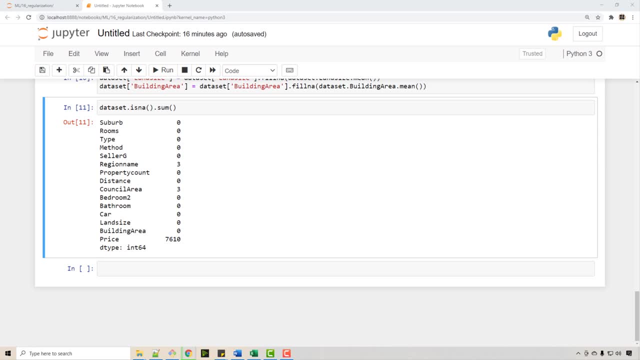 and this council leaders, I'm not going. and this council leaders, I'm not going to care about it too much now. I will to care about it too much now. I will to care about it too much now. I will drop those values. so like these three. so 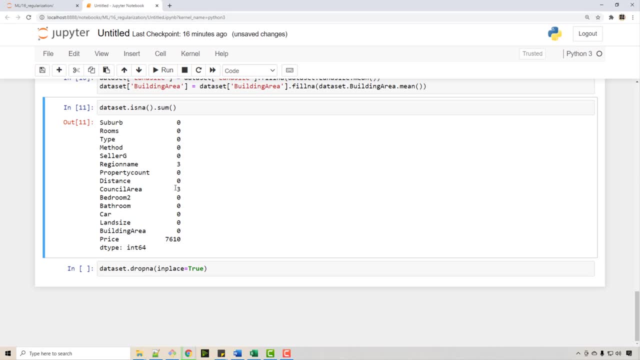 drop those values. so like these three. so drop those values, so like these three. so if you have a couple of random columns, if you have a couple of random columns, if you have a couple of random columns with any value, you can drop it. you know, with any value you can drop it, you know. 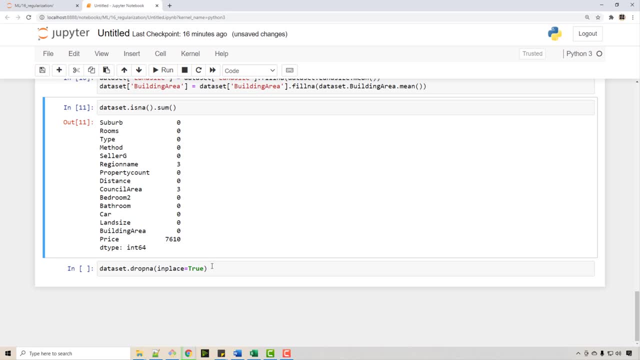 with any value, you can drop it. you know our data set is huge and if you drop, our data set is huge. and if you drop, our data set is huge. and if you drop, like these three and three, six rows, it's like these three and three, six rows, it's. 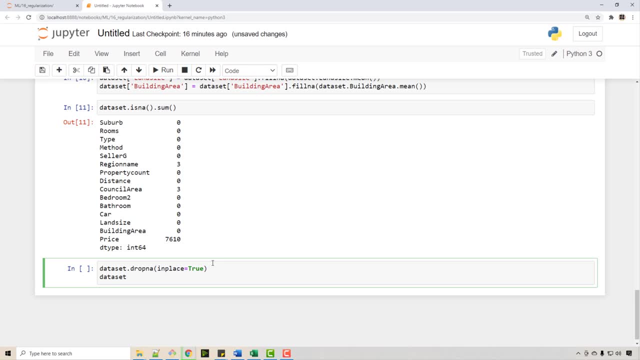 like these three and three, six rows. it's not a big deal, so I will just drop them. not a big deal, so I will just drop them. not a big deal, so I will just drop them and run the same function again and you. and run the same function again and you. 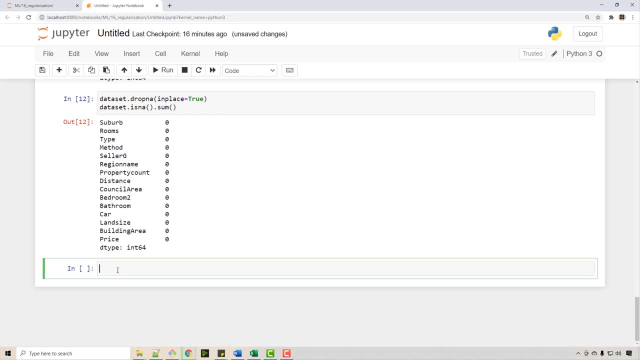 and run the same function again and you see, like none of the columns have, well see, like none of the columns have, well see, like none of the columns have, well, any values now. so now I have some any values now. so now I have some any values now. so now I have some categorical features which I want to. 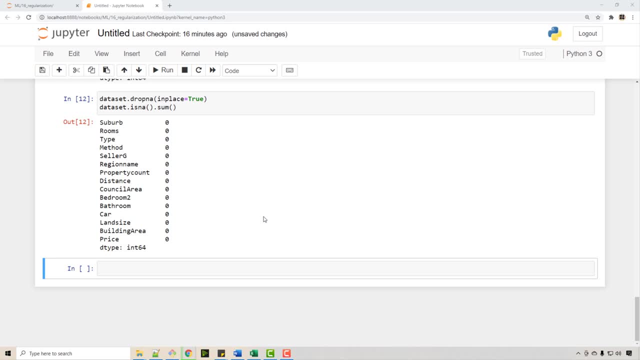 categorical features which I want to categorical features which I want to convert into dummies. you know I want to convert into dummies. you know I want to convert into dummies. you know I want to do one hot encoding so you guys might do one hot encoding so you guys might. 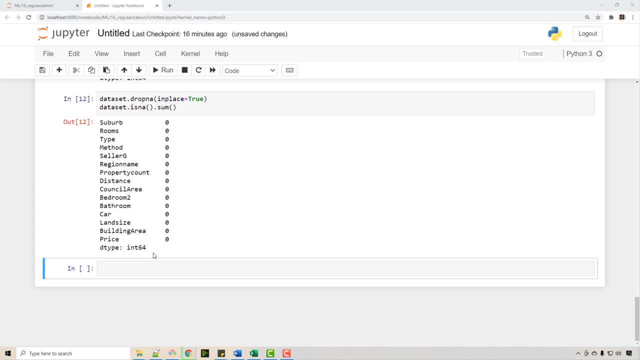 do one hot encoding so you guys might know about one hot encoding. if you don't know about one hot encoding, if you don't know about one hot encoding, if you don't, I have a one hot encoding video. so I have a one hot encoding video. so 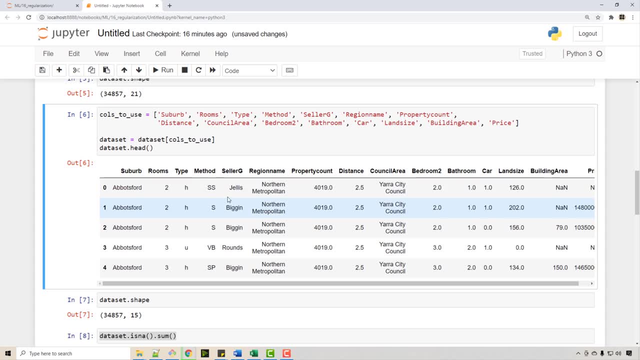 I have a one hot encoding video. so things like sub up, for example: right. any things like sub up, for example, right. any things like sub up, for example, right. any text column that you have, you need to do text column that you have, you need to do text column that you have, you need to do a dummy encoding and pandas provide a. 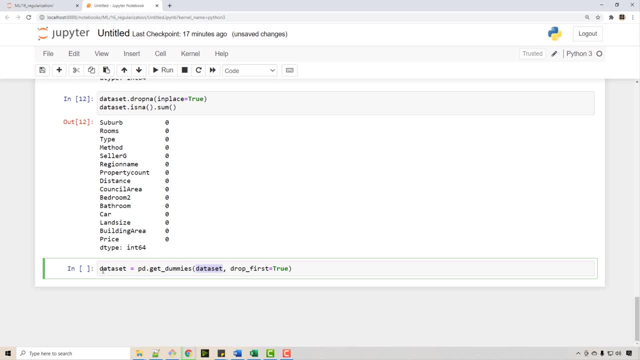 a dummy encoding and pandas provide a a dummy encoding and pandas provide a very convenient API called get dummies. very convenient API called get dummies. very convenient API called get dummies. so from data set, you get this and you. so, from data set, you get this and you. 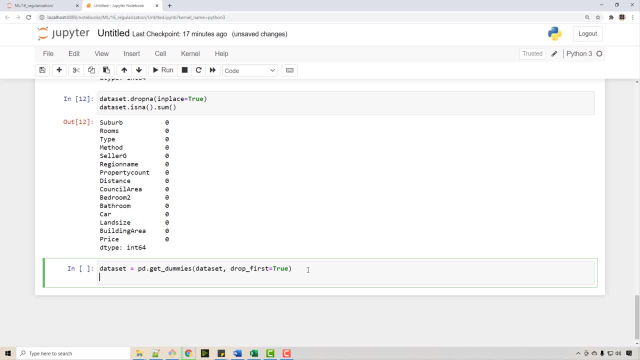 so from data set you get this and you drop first, because you want to avoid the drop first, because you want to avoid the drop first, because you want to avoid the dummy variable trap again. if you don't dummy variable trap again, if you don't dummy variable trap again, if you don't know about dummy variable trap, you can. 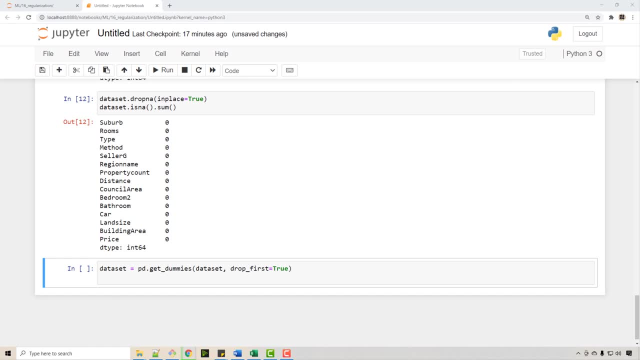 know about dummy variable trap. you can know about dummy variable trap. you can watch my one hot encoding video and watch my one hot encoding video and watch my one hot encoding video and this will kind of drop that first column. this will kind of drop that first column. 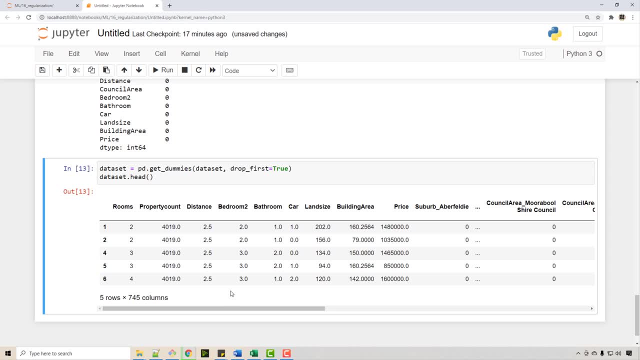 this will kind of drop that first column. when you do it encoding, so now when I. when you do it encoding, so now when I. when you do it encoding, so now when I look at my data set, you see everything. look at my data set, you see everything. 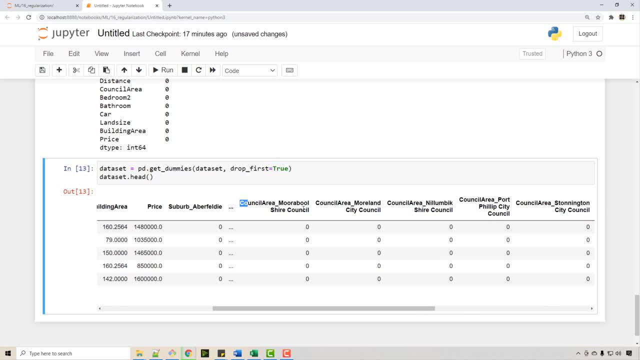 look at my data set, you see everything. there's no text column. and if you look, there's no text column. and if you look, there's no text column. and if you look at this council, it as a council area. at this council, it as a council area. 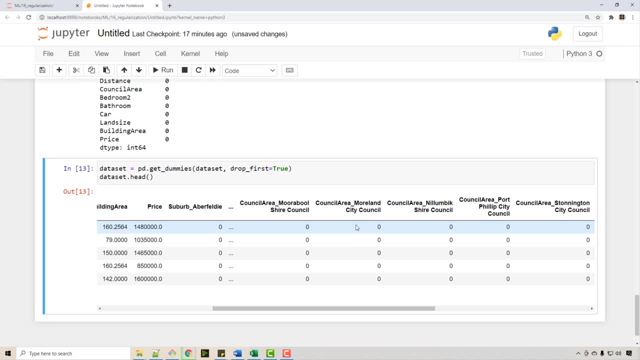 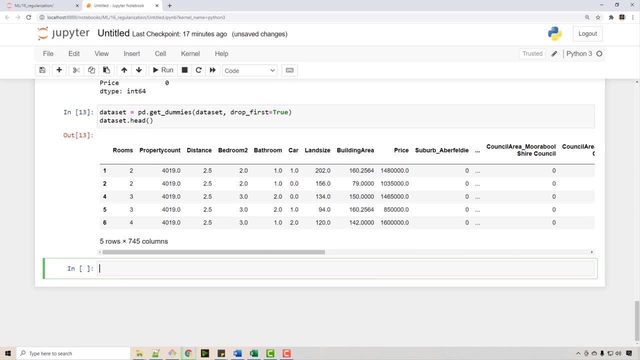 at this council it as a council area underscore. so it created a separate underscore. so it created a separate underscore. so it created a separate column for each of the council area. so column for each of the council area. so column for each of the council area. so this is what dummy or hot encoding. 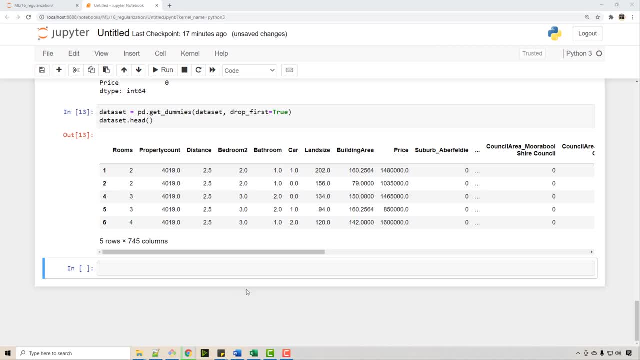 this is what dummy or hot encoding. this is what dummy or hot encoding means: now I want to create X and Y, so means now I want to create X and Y, so means: now I want to create X and Y, so my X, so I can. Y is basically price, and 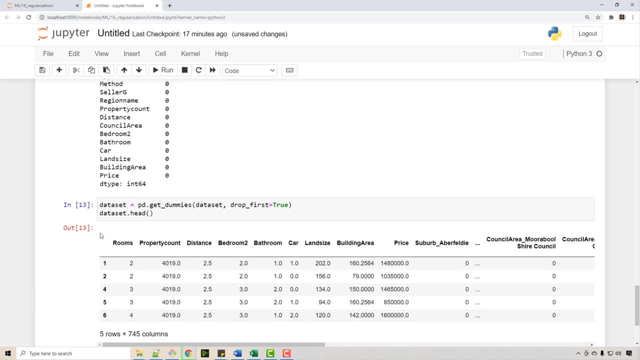 my X, so I can, Y is basically price and my X, so I can, Y is basically price and X is. you know this one? and, by the way, I had some prices as any. and, by the way, I had some prices as any. and, by the way, I had some prices as any and when I did drop any, the prices, those 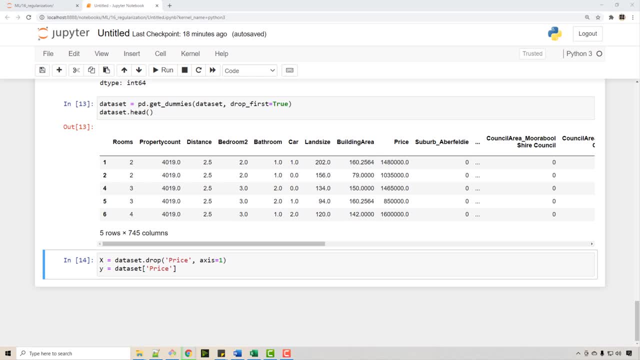 and when I did drop any, the prices those. and when I did drop any, the prices those, any values got dropped as well. so my any values got dropped as well, so my any values got dropped as well. so my data set looks pretty good and I will do. 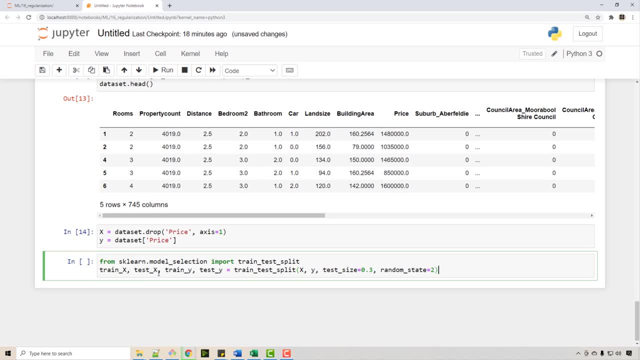 data set looks pretty good and I will do. data set looks pretty good and I will do. now train test split, so train test split. now train test split, so train test split. is this, all of these are like standard? is this, all of these are like standard? is this, all of these are like standard, usual methods? we have code in previous 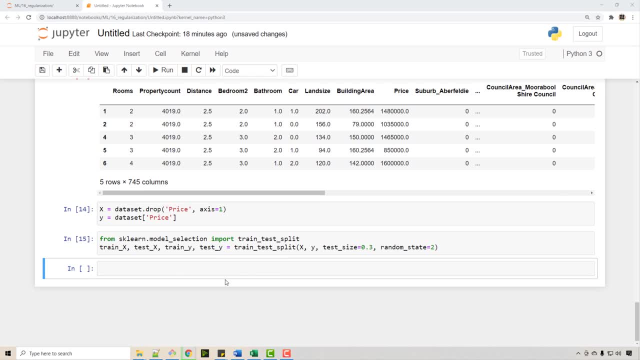 usual methods. we have code in previous usual methods. we have code in previous video. that's why I'm kind of going over video. that's why I'm kind of going over video. that's why I'm kind of going over it a little fast. you are doing a 30%. 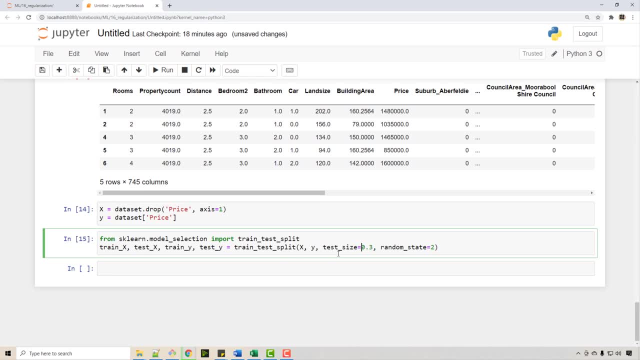 it a little fast. you are doing a 30% it a little fast. you are doing a 30% split, so 30% test, 70% training. and you split so 30% test, 70% training, and you split so 30% test, 70% training, and you get all these different data sets. now we 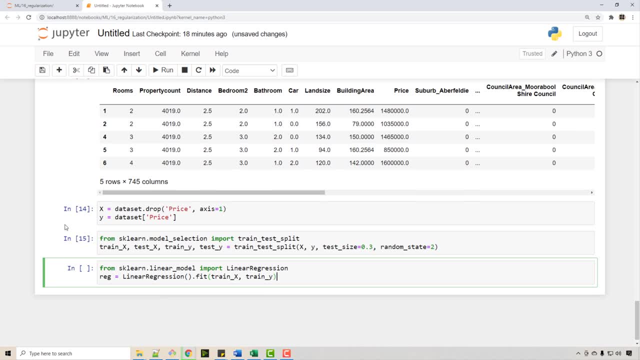 get all these different data sets. now we get all these different data sets. now we will use our regular linear regression. will use our regular linear regression. will use our regular linear regression. okay, so this is how you do regular linear. okay, so this is how you do regular linear. 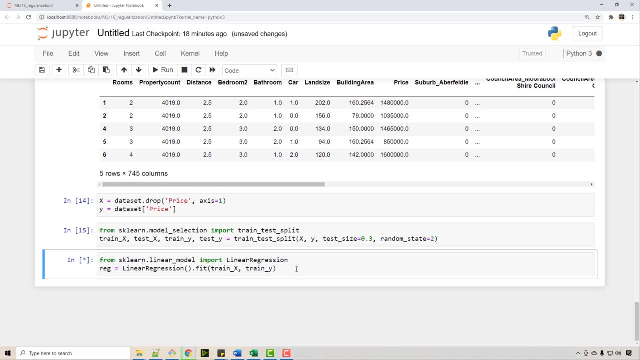 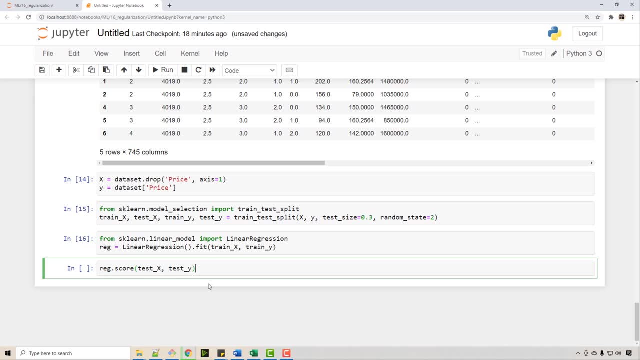 okay, so this is how you do regular linear regression, and then when you run this regression, and then when you run this regression, and then when you run this, it's gonna do training and model is fit, it's gonna do training and model is fit, it's gonna do. training and model is fit now. now I will do the score on X taste. 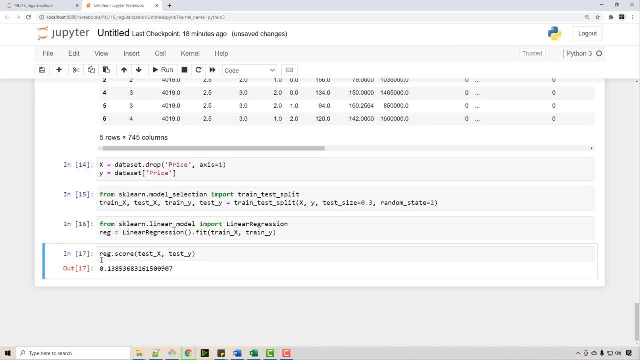 now. now I will do the score on X taste now. now I will do the score on X taste and y taste. you realize that my score and y taste. you realize that my score and y taste. you realize that my score comes out to be really low, 14%, which is. 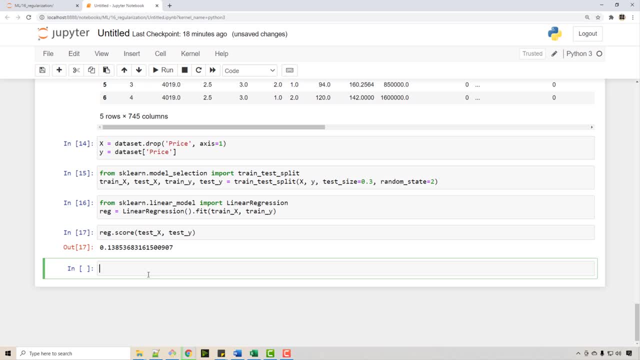 comes out to be really low 14%, which is comes out to be really low 14%, which is very, very low score. but if you do a very, very low score, but if you do a very low score, but if you do a score on training, data set say it is 68%. so 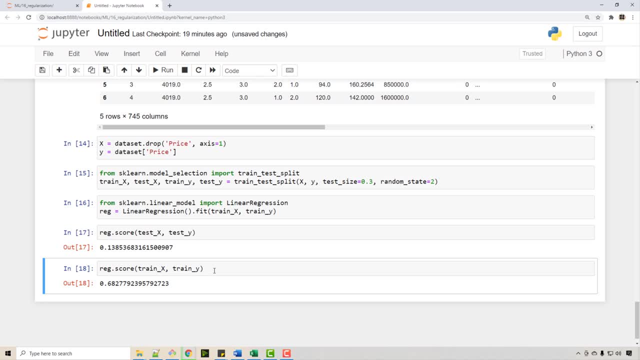 score on training data set, say it is 68%. so score on training data set: say it is 68%. so this is clearly overfitting your. this is clearly overfitting your. this is clearly overfitting your data set. your data set was so much. 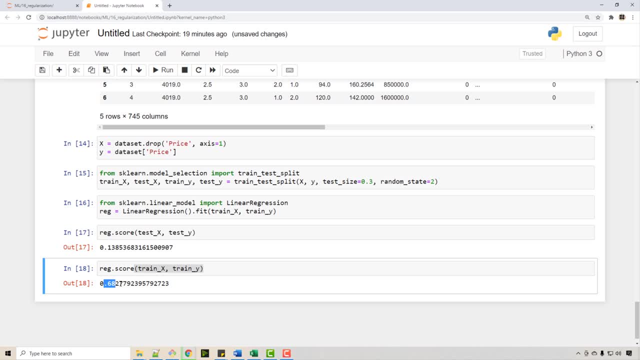 data set. your data set was so much data set. your data set was so much overfit that for training samples. it overfit that for training samples. it overfit that for training samples. it gave a good accuracy but for taste. gave a good accuracy, but for taste. 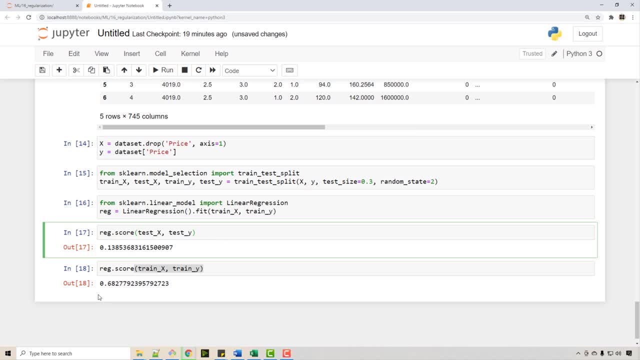 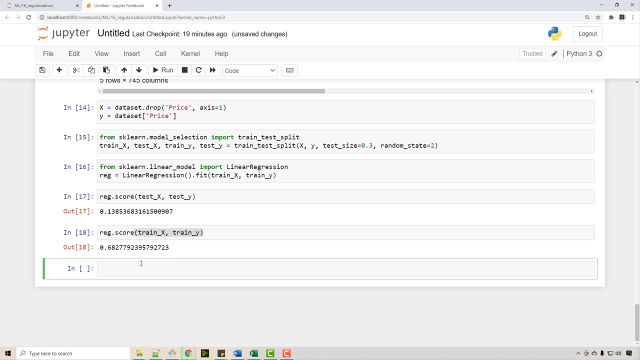 gave a good accuracy, but for taste samples, the data samples that it has not. samples the data samples that it has not. samples the data samples that it has not seen before. it gave a horrible score, so seen before it gave a horrible score, so seen before it gave a horrible score. so how do you address this? SK learn. 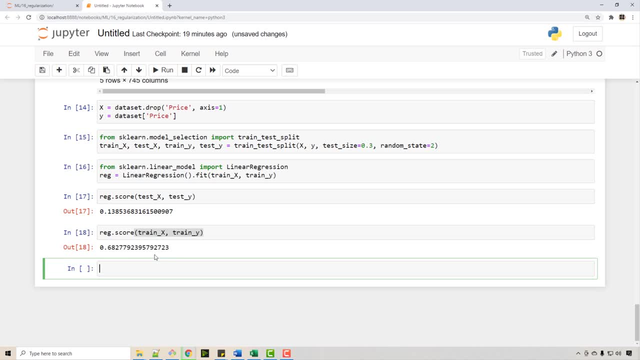 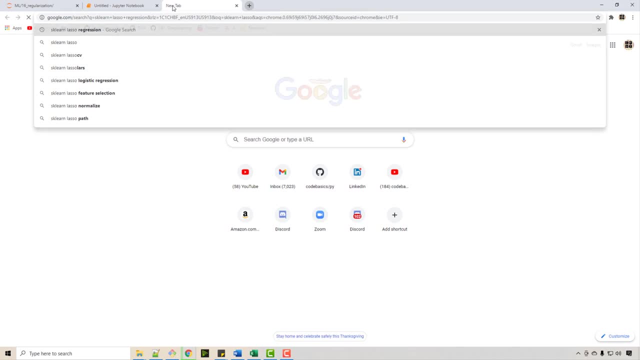 how do you address this SK? learn. how do you address this SK? learn lasso regression is basically l1 lasso regression is basically l1 lasso regression is basically l1 regularization. so if you do SP, learn regularization. so if you do SP, learn regularization. so, if you do SP, learn lasso recreation. 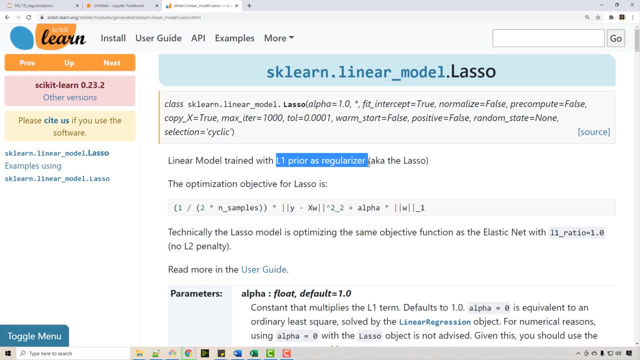 lasso regression. lasso regression: see, this is the lasso regression and it see, this is the lasso regression and it see, this is the lasso regression and it is l1 regularization, so I am going to is l1 regularization, so I am going to. 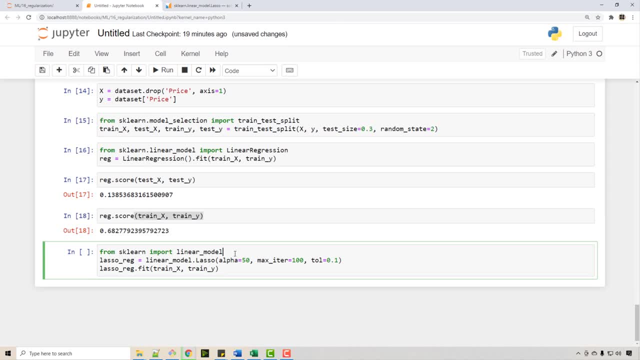 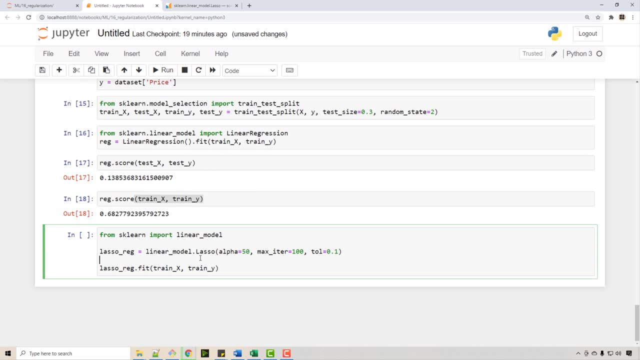 is l1 regularization, so I am going to use that model, use that model, use that model. so I created a model, imported that, and so I created a model, imported that. and so I created a model, imported that, and then I created a lasso regression object. then I created a lasso regression object. 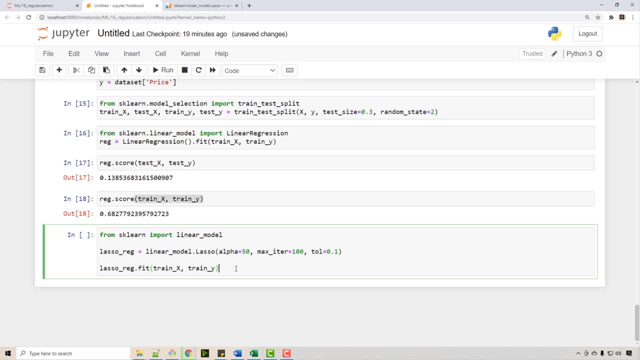 then I created a lasso regression object with alpha. well, I'm initializing with alpha. well, I'm initializing with alpha. well, I'm initializing this alpha value to be random. you can this alpha value to be random. you can this alpha value to be random. you can play with these values and see which one. 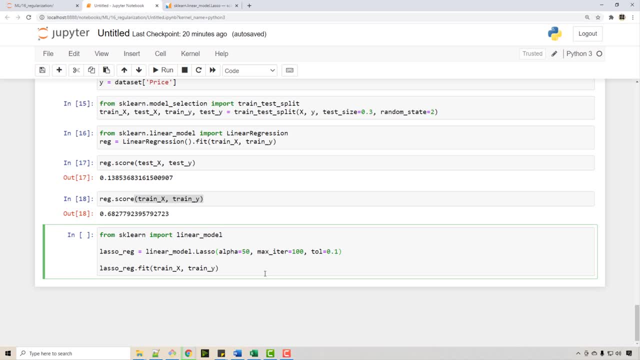 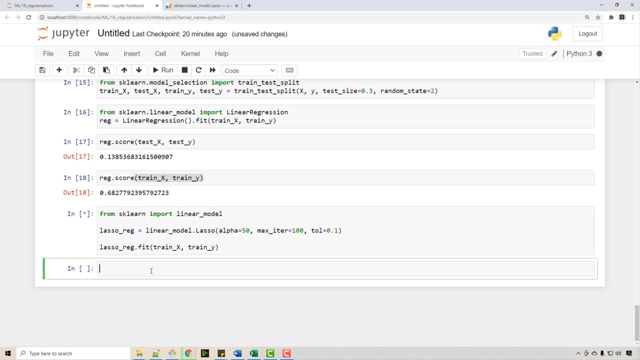 play with these values and see which one play with these values and see which one gives you a better accuracy. and I gives you a better accuracy and I gives you a better accuracy and I initialize few other parameters as well. initialize few other parameters as well. initialize few other parameters as well. and when I now run my regression, it is: 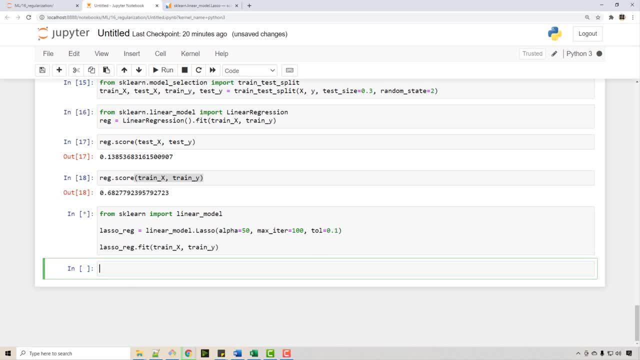 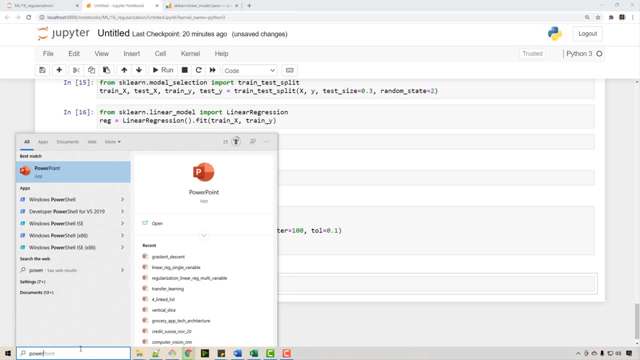 and when I now run my regression, it is. and when I now run my regression, it is fitting it with the regularization, fitting it with the regularization, fitting it with the regularization parameter on. so if you look at our parameter on so, if you look at our parameter on so, if you look at our equation earlier. so let me open our. 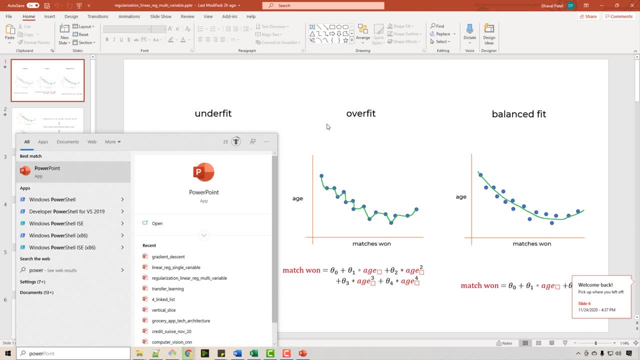 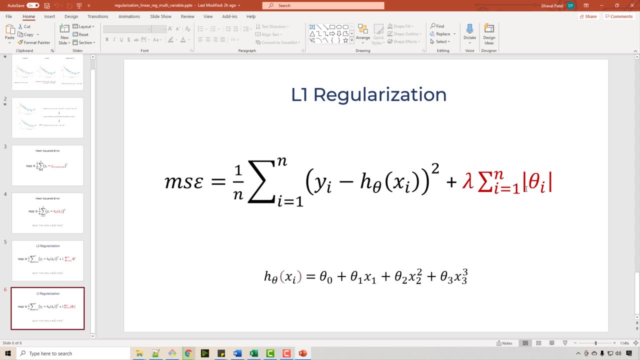 equation earlier, so let me open our equation. in that equation, L1 regularization will add an absolute L1 regularization will add an absolute L1 regularization will add an absolute theta value in your error. and this is the theta value in your error and this is the theta value in your error and this is the formula it will use during the 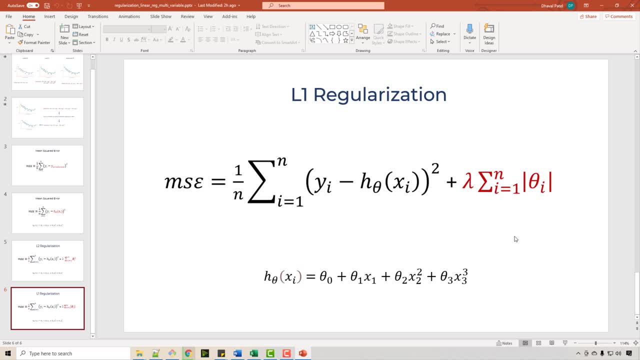 formula it will use during the formula it will use during the training: simple linear regression without any training. simple linear regression without any training. simple linear regression without any regularization will not have this red regularization, will not have this red regularization, will not have this red parameter. so that's the only difference. 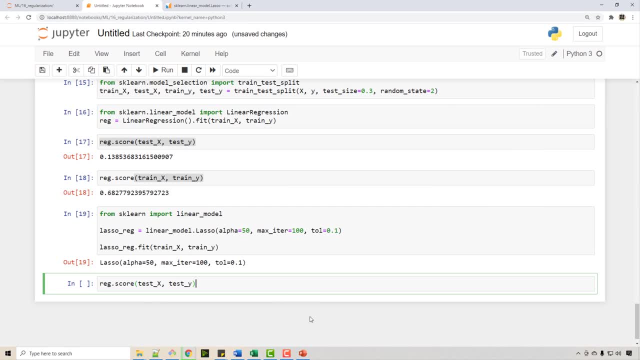 parameter. so that's the only difference parameter. so that's the only difference. now let's do a score on your test. now let's do a score on your test. now let's do a score on your test. so I will do lasso regression score. and so I will do lasso regression score and. 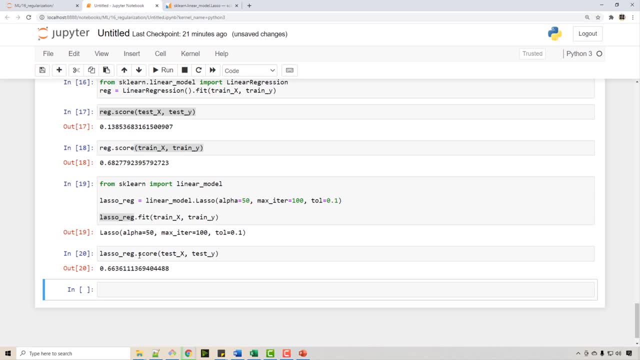 so I will do lasso regression score and you find that accuracy improved and I, you find that accuracy improved and I, you find that accuracy improved and I, just to make sure, I will also do a score, just to make sure I will also do a score, just to make sure, I will also do a score on X taste and on training as well. so 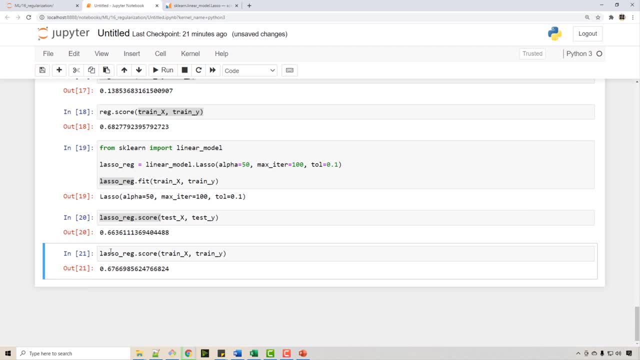 on X taste and on training as well. so on X taste and on training as well. so you see, training and taste. both are you see, training and taste. both are you see, training and taste. both are giving a very good, not very good, but 67, giving a very good, not very good, but 67. 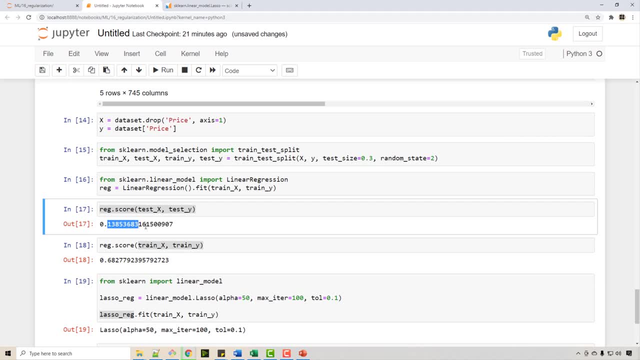 giving a very good- not very good, but 67 percent accuracy, which is compared to 13 percent. accuracy, which is compared to 13 percent. accuracy, which is compared to 13 percent. it improved to 66 percent. you percent. it improved to 66 percent. you percent. it improved to 66 percent. you can see how much of a big difference our 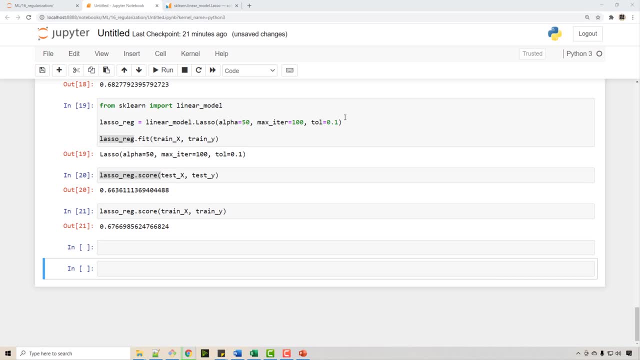 can see how much of a big difference our can see how much of a big difference our regularization can make. there is L2 regularization can make. there is L2 regularization can make. there is L2 regularization as well, and it's called regularization as well and it's called. 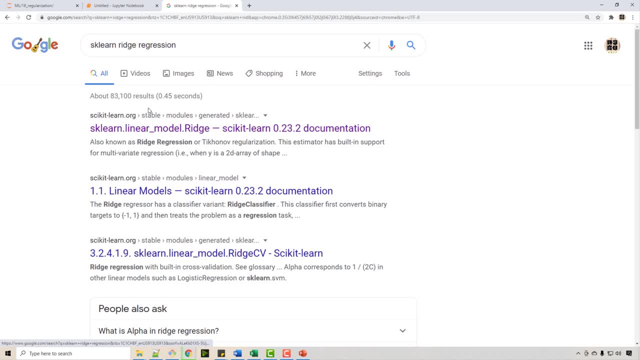 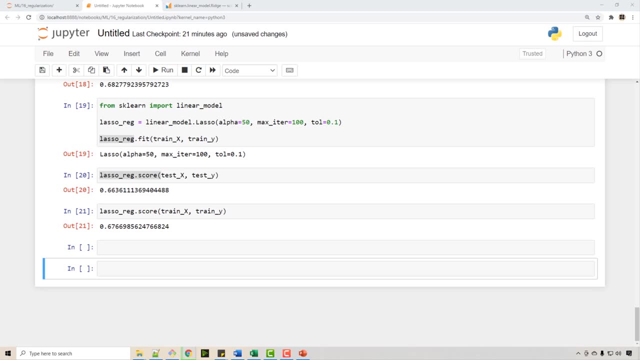 regularization as well, and it's called ridge regression. so if you do a scale on ridge regression, so if you do a scale on ridge regression, so if you do a scale on ridge regression, this one is an L2 ridge regression, this one is an L2 ridge regression, this one is an L2 regularization, and here I can import that. 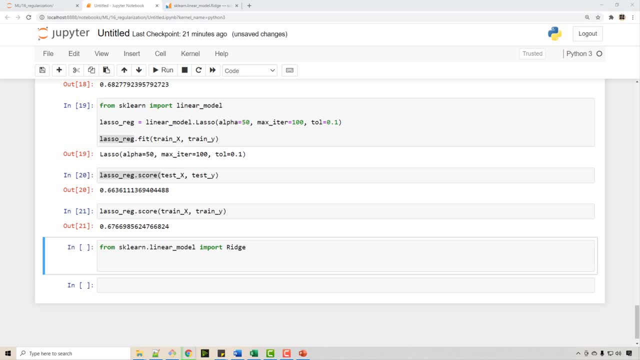 regularization. and here I can import that regularization. and here I can import that from a scale on library. as usual, I, from a scale on library. as usual, I from a scale on library. as usual, I create a region integration class object. create a region integration class object. create a region integration class object which will look like this and call a fit. 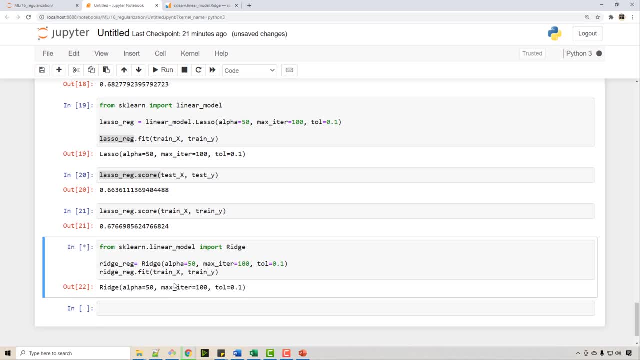 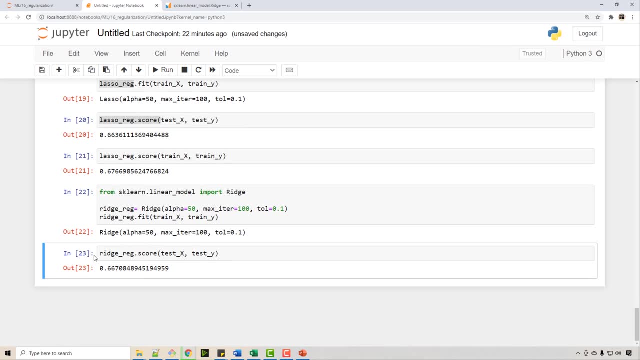 which will look like this and call a fit, which will look like this and call a fit method on this method, on this method, on this, and then when I do a score on your test, and then when I do a score on your test, and then when I do a score on your test, data set, it looks again: it's 67%. so 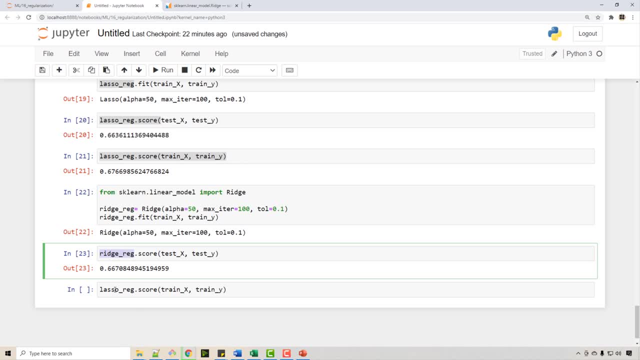 data set: it looks again: it's 67%. so data set: it looks again it's 67%. so it's pretty good and let's check on it's pretty good. and let's check on it's pretty good and let's check on training data set. training data set is. 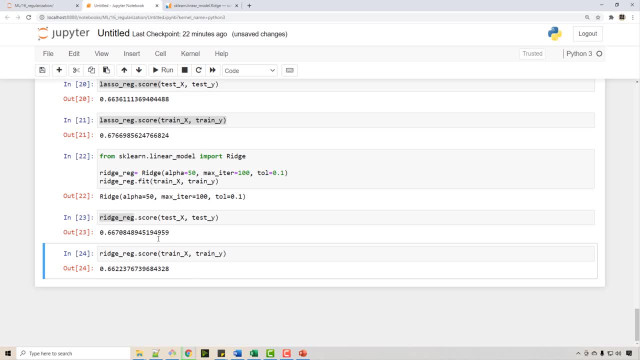 training data set. training data set is training data set. training data set is also. you know it's pretty pretty good also. you know it's pretty pretty good also. you know it's pretty pretty good. so you saw that by using ridge. so you saw that by using ridge. 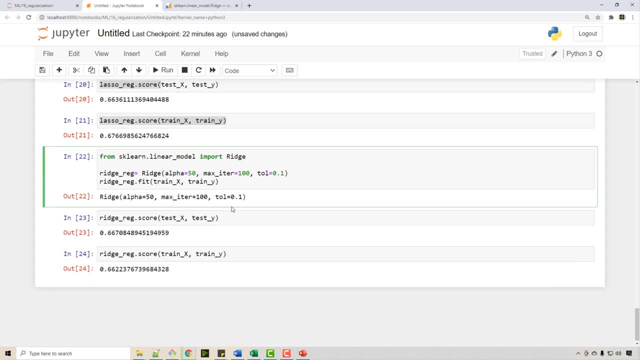 so you saw that by using ridge regression and lasso regression. so ridge regression and lasso regression. so ridge regression and lasso regression. so ridge is L2, lasso is one your accuracy for is L2, lasso is one your accuracy for is L2 lasso is one your accuracy for your not seen data samples, which is your. 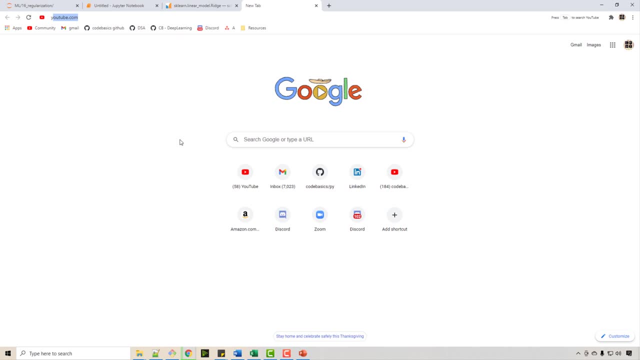 your not seen data samples, which is your? your not seen data samples, which is your? test sample improved a whole lot. if you test sample improved a whole lot. if you test sample improved a whole lot. if you are trying to learn machine learning, you are trying to learn machine learning you. 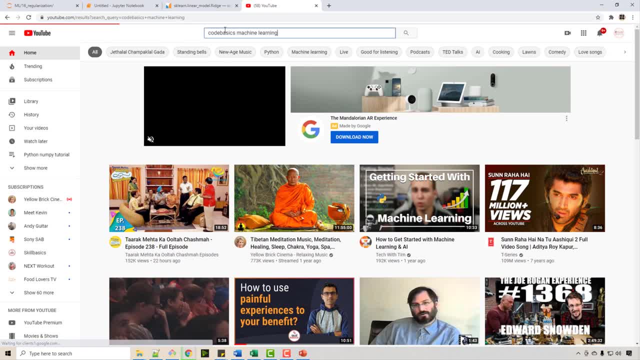 are trying to learn machine learning. you can just in YouTube, you can just search. can just in YouTube, you can just search. can just in YouTube, you can just search. code basics: machine learning tutorials. code basics- machine learning tutorials. code basics- machine learning tutorials. I have the complete list of machine